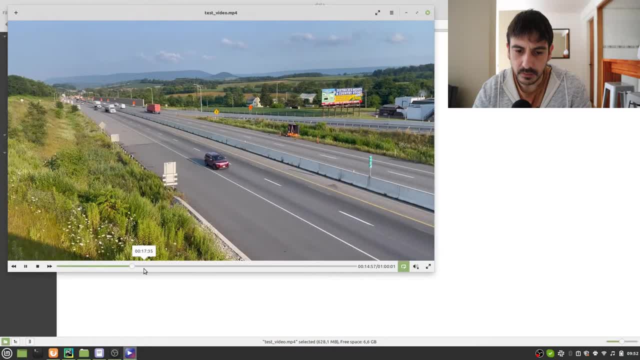 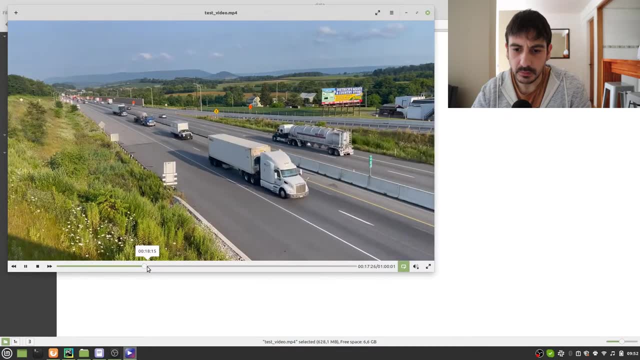 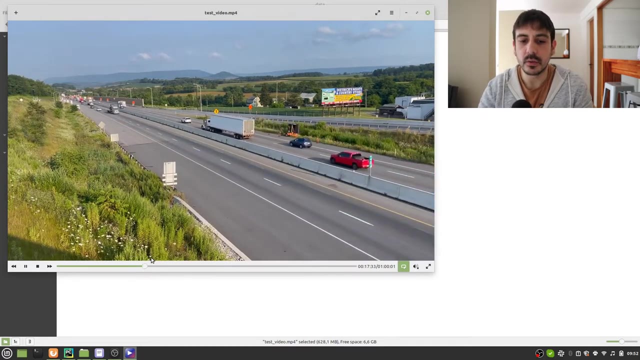 going to choose a section of this video. i have already been looking at this video and this is a section that i think is going to be interesting because there are many different objects going around, so i am going to split a 20 seconds video, which is centered: 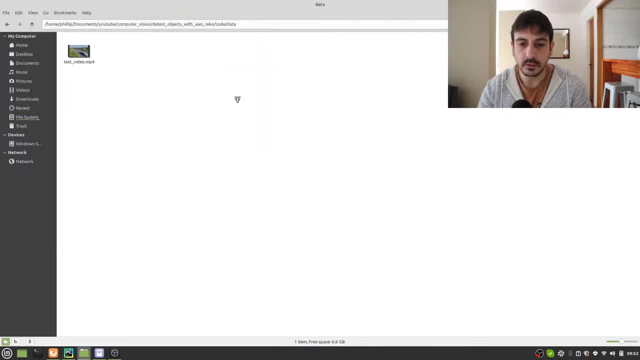 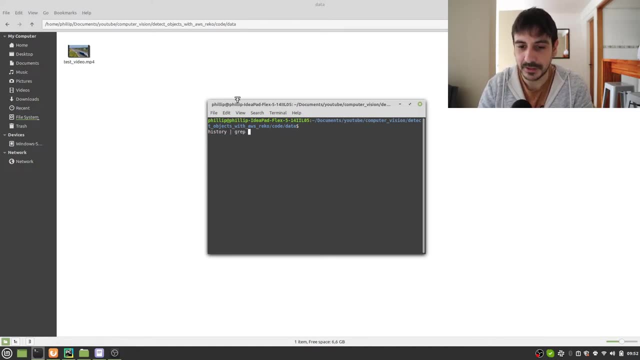 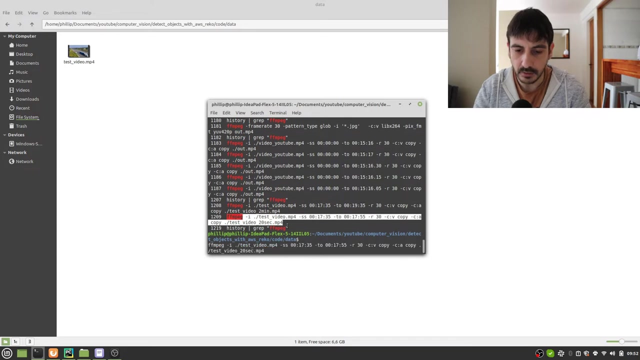 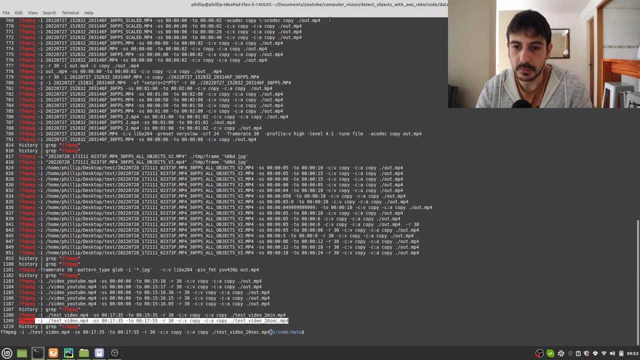 around this location and i'm going to call ffmpeg. i have i'm. i have the command ready to be used. if i look for ffmpeg, you can see. when i was preparing this video i have already used this command and basically what i am doing in this ffmpeg command. let me clear. 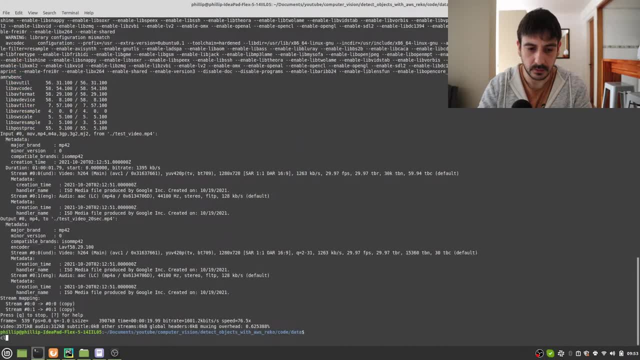 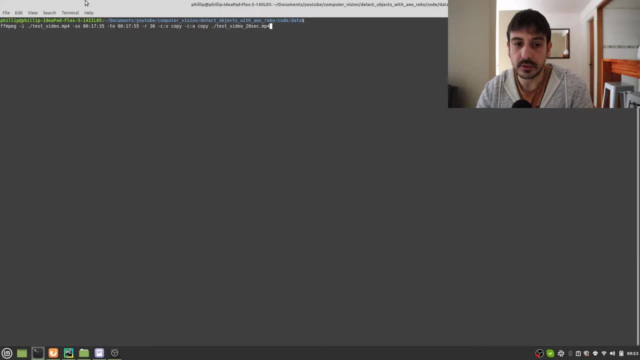 let me execute it and then i will clear the terminal. what i am doing in this command is calling the video which i just showed you- the one hour long video- and to splitting this video in only a 20 seconds video. you can see from the minute 1735 to 1755. 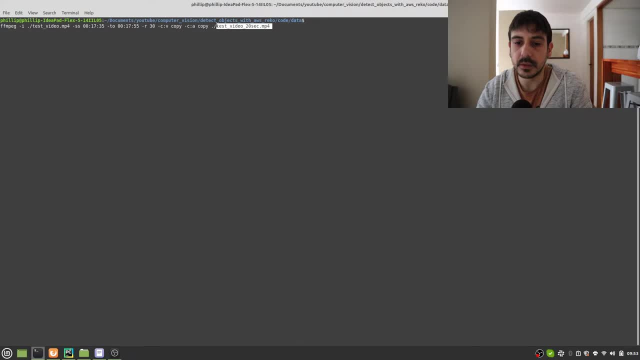 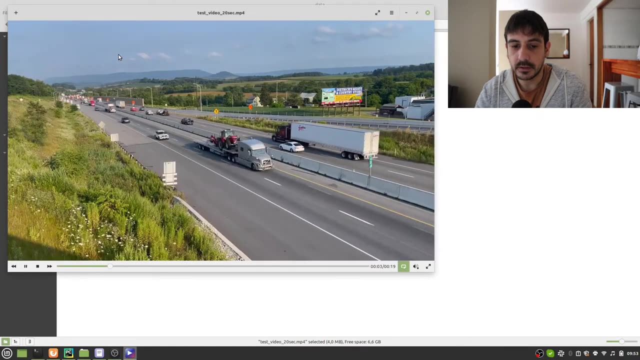 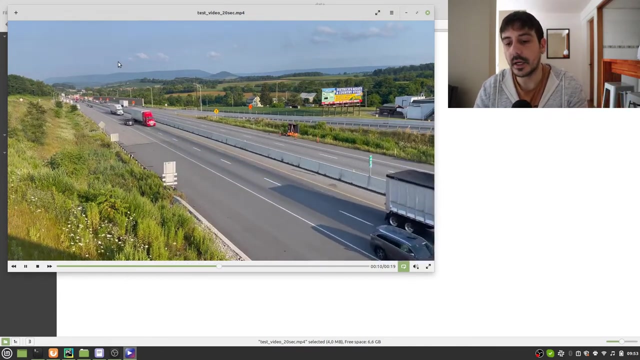 and i am creating a new video from it which is called test video, 20 seconds, mp4. you can see this is the video i have just created and this is the video i am going to use to detect objects. it's just like a 20 seconds video from my original video, and i split this video. 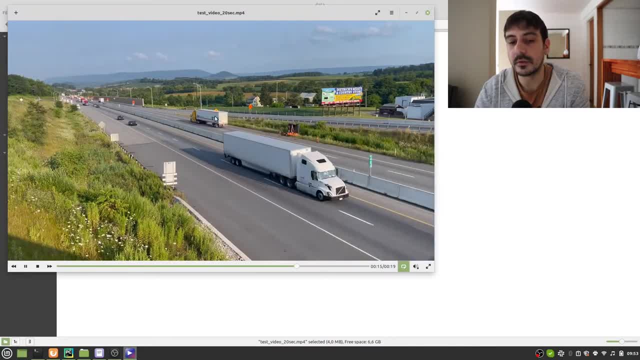 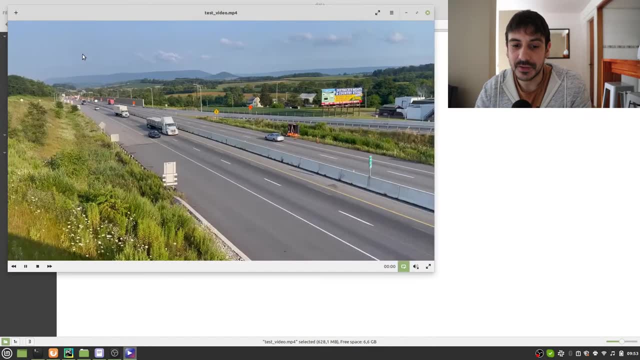 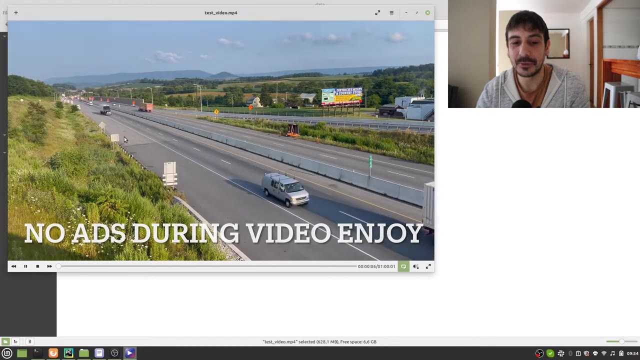 only by looking at a section with a lot of different cars and objects and tracks and so on, because in this one hour long video there are some times where there's absolutely nothing going on and it would be super boring to show you how the object detector works in an empty highway. 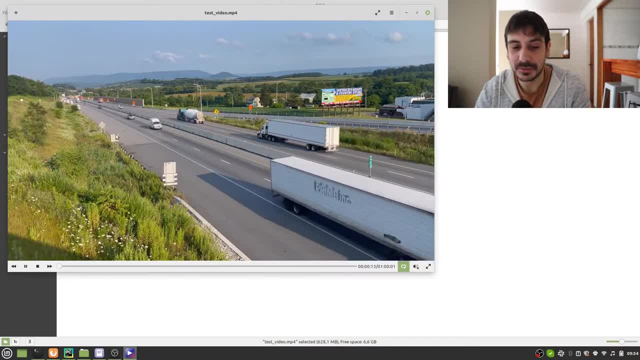 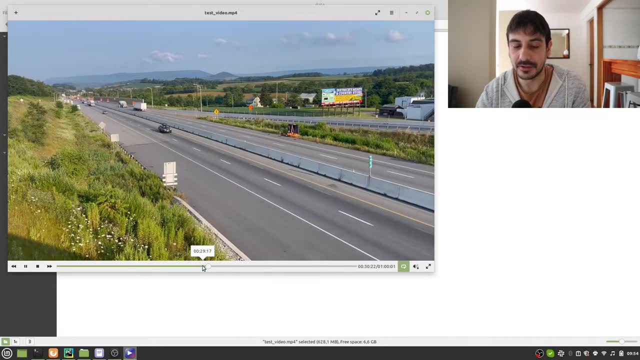 with absolutely no cars and tracks and so on. uh, trust me, i have been looking at some sections of this video and there are some times where there's nothing going on. for example, here there are only a few cars, but anyway. so we are going to work in this 20 seconds. 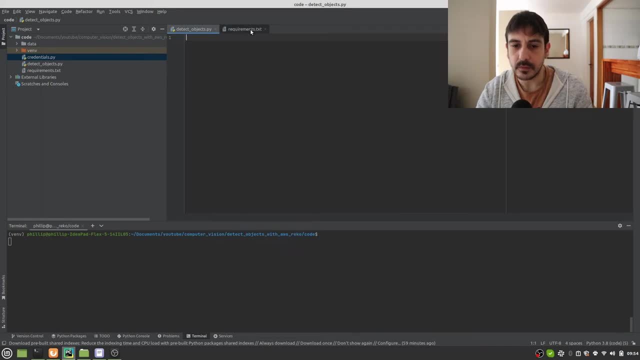 video, and let's start with it. i have created this requirements file. these are the dependencies we are going to use in this tutorial and it's basically bottle 3, which is the library we are going to use to communicate with amazon, then opencv and matlab divs. so what i am going to do. 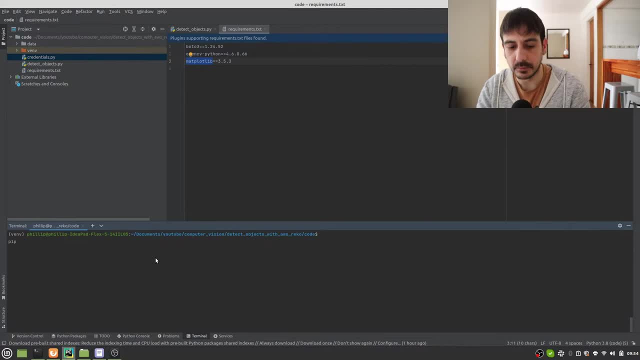 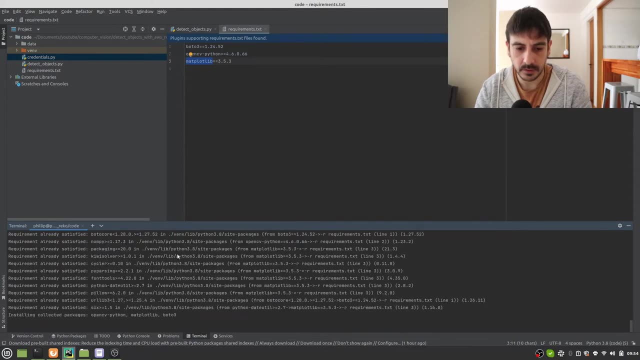 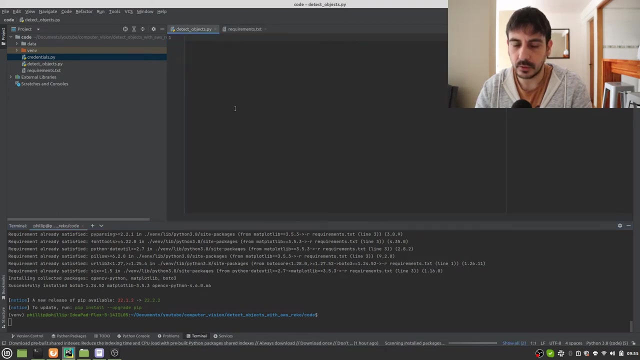 i have already created my virtual environment and i have activated my virtual environment. i'm going to pip install these dependencies. okay, everything has been installed, so i am going to code in this script. so the first thing i'm going to do is to import all the needed libraries. 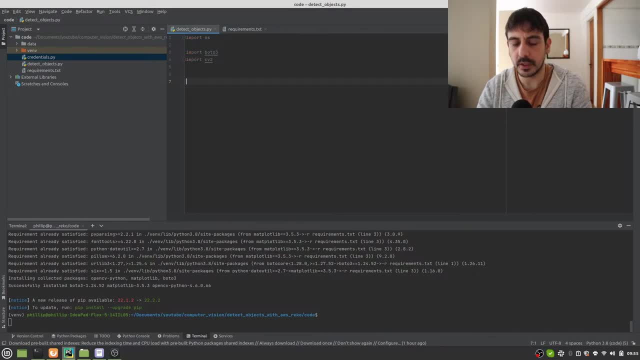 and cv2. okay, i'm going to do is to create an object which is going to be called. this is the file i am going to use. so input file is located in data and then this is the file name we are going to use. what i am going to do is iterating in all the frames. 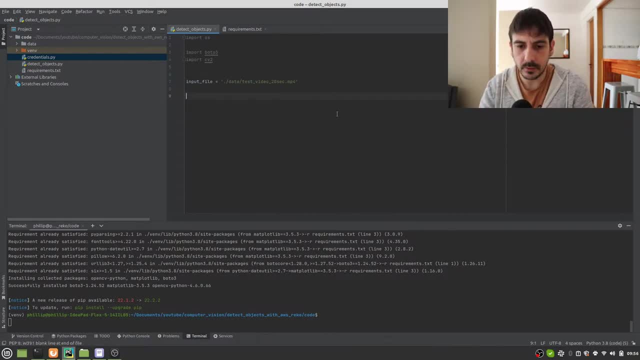 from this 20 seconds video. so what i am going to do now is to create an object which is going to be cap- and cap is equal to cv2 video capture- and then my input file for my input video. so what i'm doing here is to create, creating an object which is going to represent my video. 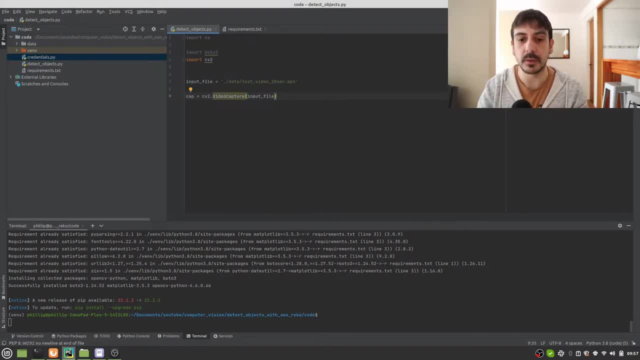 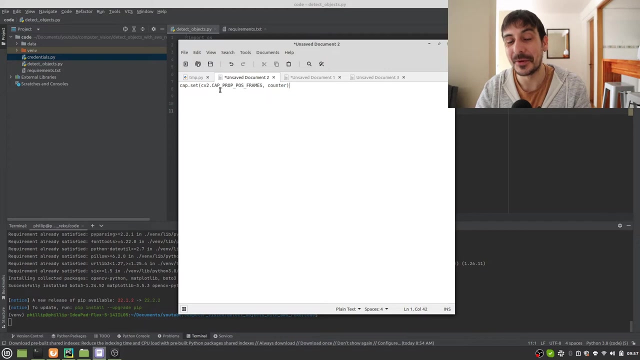 or is the object i am going to use to extract frames from my video. so i have created this object and then i have to call the, an additional command which is going to extract all the frames from my video. this is a command i never remember, so when i was preparing this video, i copy pasted. 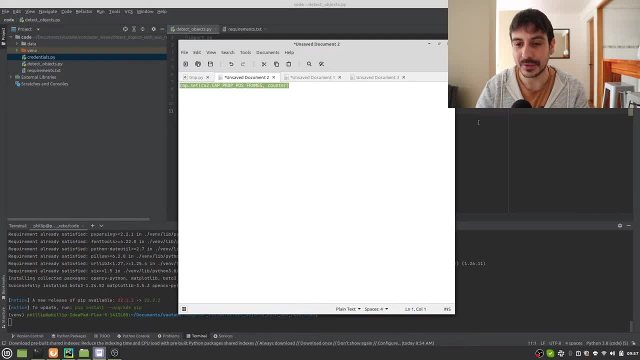 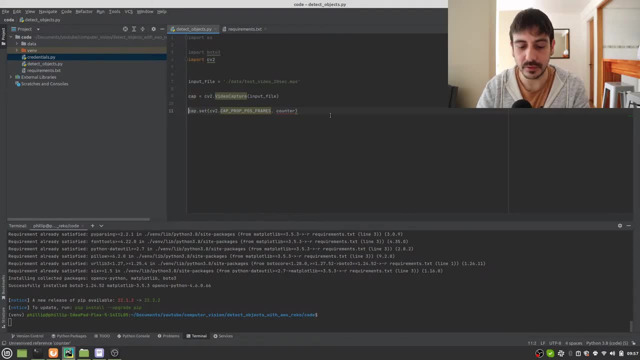 this instruction, so it's ready to be used. so this is the um, the command we are going to use in order to extract frames. this is going to be equal to red frame, and for this we need a counter. so i'm going to initialize this value in zero and what i'm doing in this instruction is to extract. 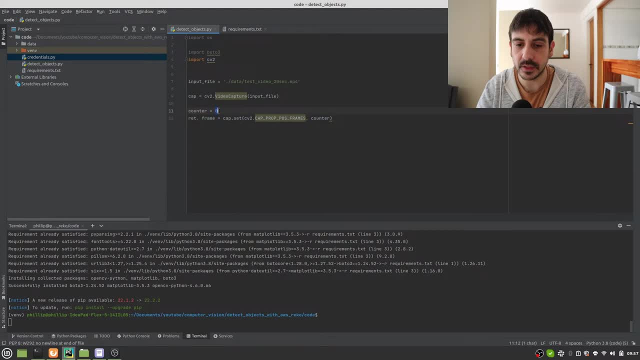 the frame number counter, then the frame number zero, in this case from the video i have created, right? so what i'm going to do is to iterate in all the frames from zero to the number of frames, and this way i'm going to extract all the frames. so let's start with it. 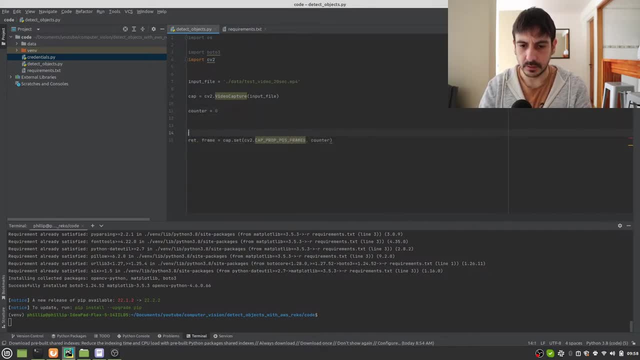 and let me do it in a different way. i'm going to do something like this: red equal true, and then, while red, i'm going to do this right. so every time there's a new frame, this value is going to be true, and if we do something like this, it's going to be enough. counter plus equal one, okay. 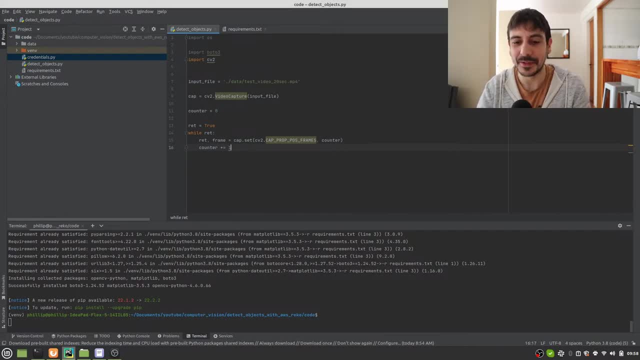 this is like the building blocks we're going to need in order to create all this process, because now we are incrementing the number of frames and we are just extracting frames, and we are going to do this while we while there are available frames to extract. so this is pretty much all we need in order to read the frames. what i'm going to do now is to 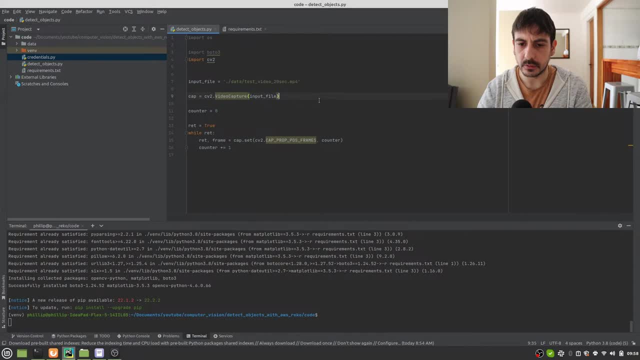 create my bottle 3 client. i'm going to create this client here. client is going to be recognition node. this is: this is record client, which is um. this is record client, which is the client we are going to use in order to communicate with a lds. 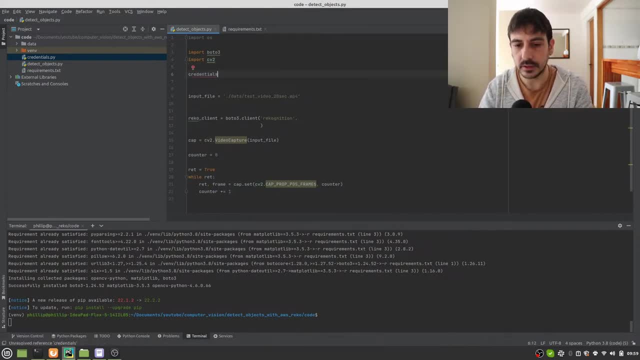 recognition and i need to give this um client two variables which are going to be my access key credentials. so in my case i have already created to call these parameters access key. sorry id, i may be making a mistake. i'm going to take a closer look in a few minutes. and then is 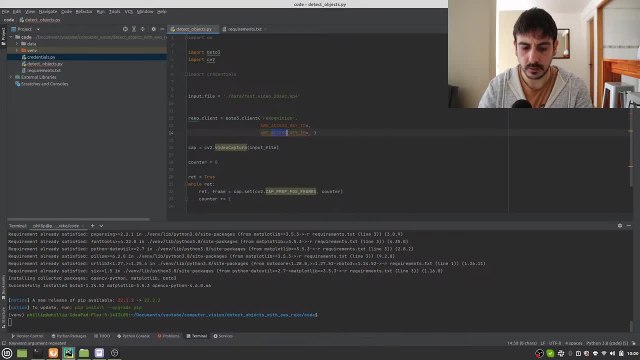 the secret key, which is something like this: this may not be exactly the right values- i'm going to take a look in a couple of minutes- but it's basically basically that idea. so it's going to be credentials dot- access key and this is credentials dot- secret key. and if you want to, 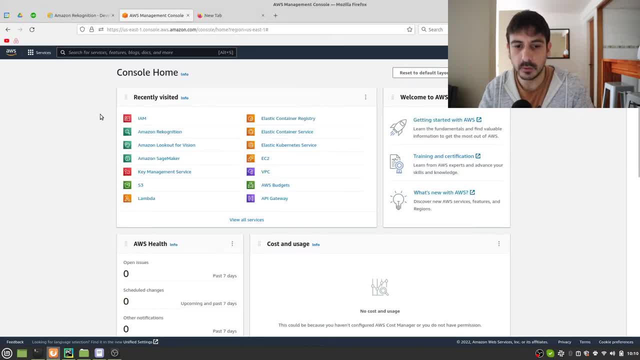 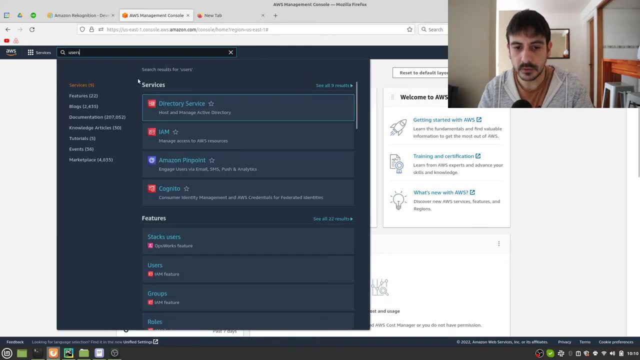 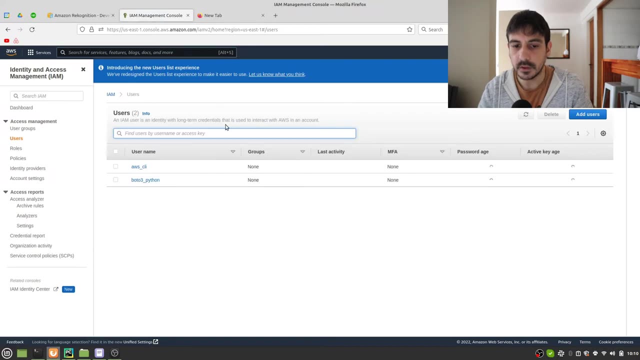 know how to get your credentials, your aws credentials. what you need to do is going to aws, to your console, and selecting users. i'm going to users, which is one of the sections of aam, and these are, for example, my users and what you will need to do in order to create a new user you can use for this and you can get. 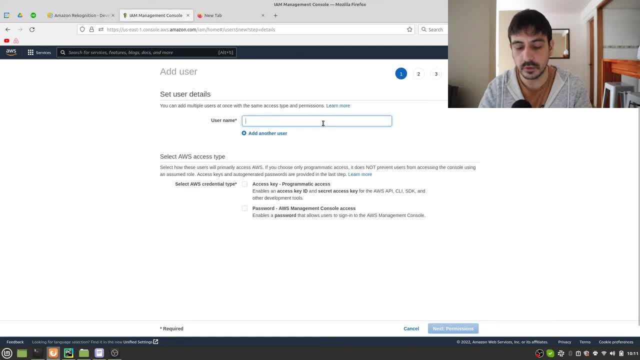 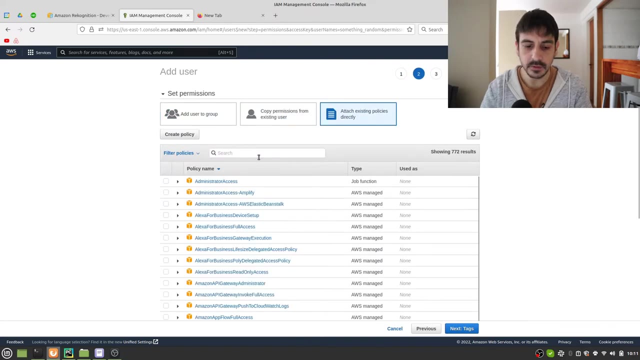 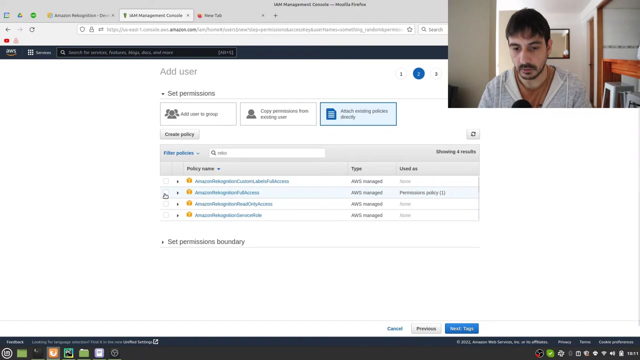 your credentials is add users. i'm just going to show you an example. this could be something, something random. i'm just going to call this user nothing and select aws credential type. this is the option you need to select, then permissions, then attach existing policies and, as you need to communicate with aws reco, you are going to look for aws amazon recognition full. 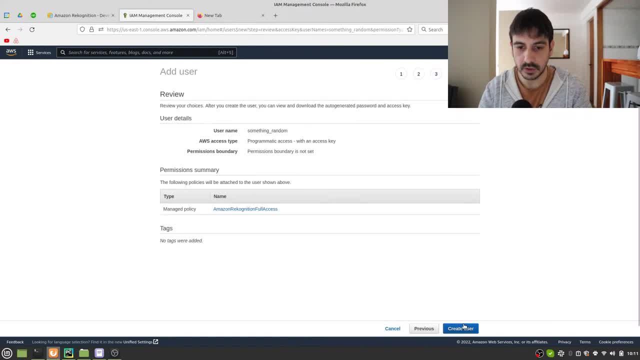 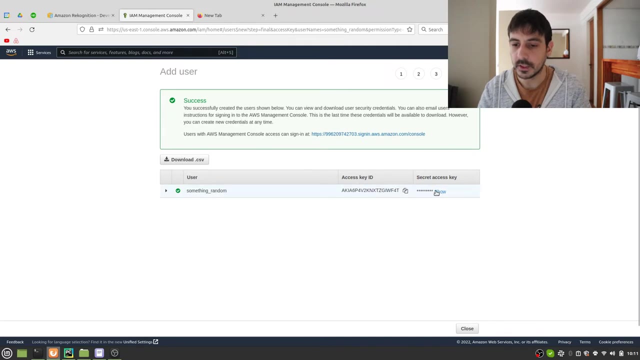 access next, and that's going to be pretty much it, if i remember correctly. yes, all we are doing is just communicating with lus, with aws, reco, so this is going to be enough. and once you do it, you are going to get these two values: this access key id and then this secret key- secret access key. 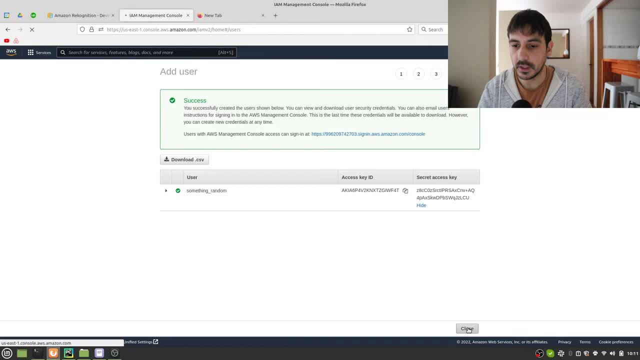 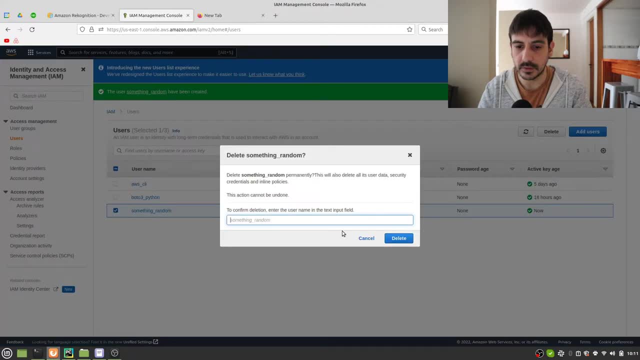 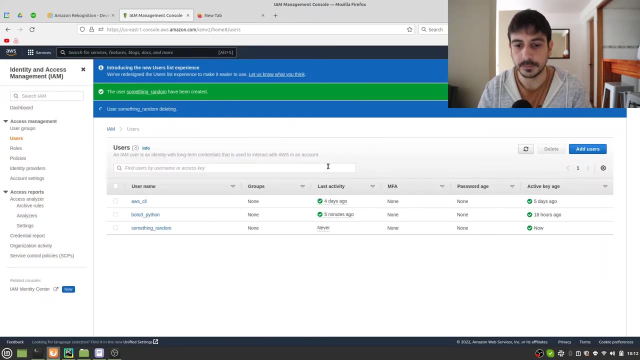 so yeah, that's pretty much how you can create a new user and in my case, i have created this user and, before i forget, i'm going to delete it because i'm not going to use it, something round, okay, so now let's back to our code. okay, so, 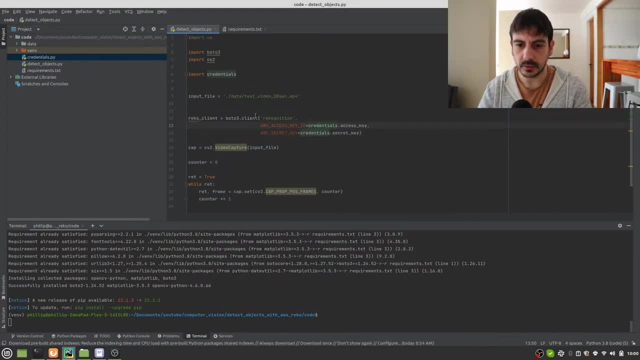 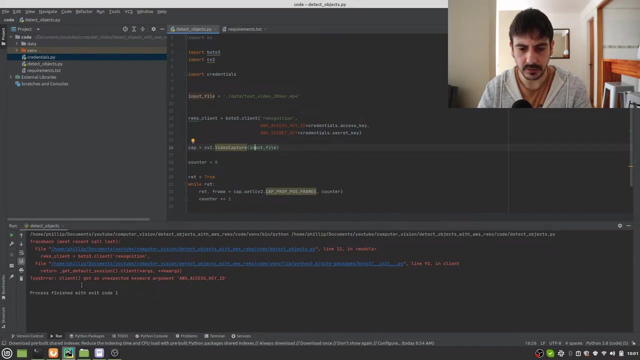 let's just execute this code it is so i can test if this client is created correctly and, if i can, can extract all the frames from my video. so for now, all i'm doing is to. it's nothing. it's just executing this command and there's something that's not right: unexpected keyword argument, let. 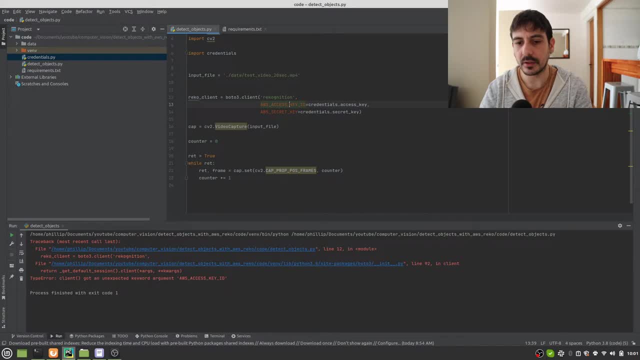 me take a look. what's the right name? oh, i see the values are okay, the numbers are okay, but i got confused and this is a lowercase, so it's something like this, it seemed. it seems my memory was uh, playing some tricks or something like that, so i'm just going to delete it and i'm going to 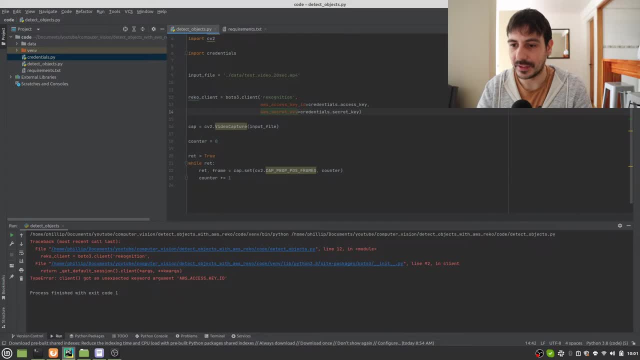 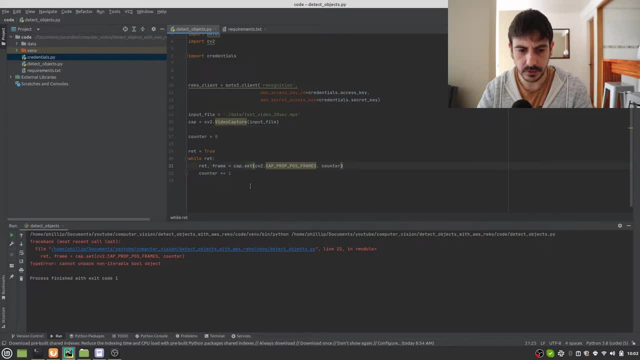 counter 0 and this should be okay. cannot unpack non-interruptible full object. oh, i see what was the problem. i had to read the frame and this red object in a different instruction. after executing, read anyway, this is just a detail. now we are connected to aws reco and we are also extracting. 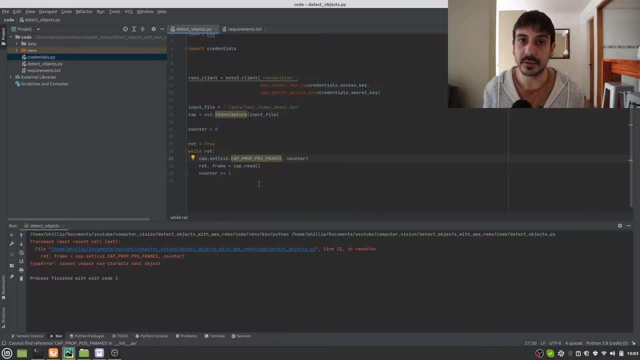 frames from our video. this is, trust me, 90 of all the process, so everything is pretty much ready. all we have to do now is just to communicate with aws, with reco and to detect the objects. so the way i am going to do this, once i have my frame, is to call reco, client dot, detect labels. 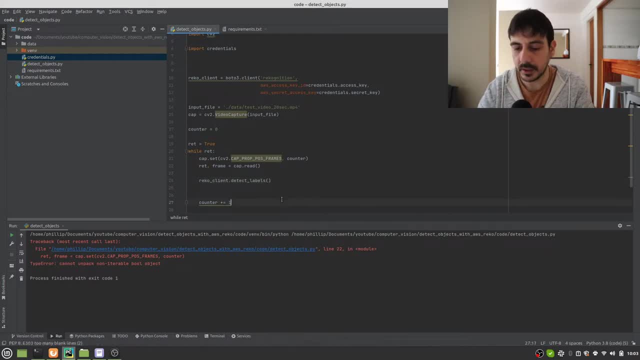 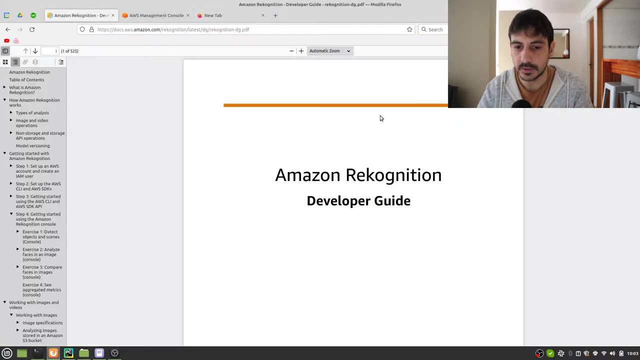 and here i'm going to give it my frame, but i have to format it in a special way and in order to that, i'm going to show you how to do it in the documentation. this is amazon recognition developers guide and if i look for detect labels, 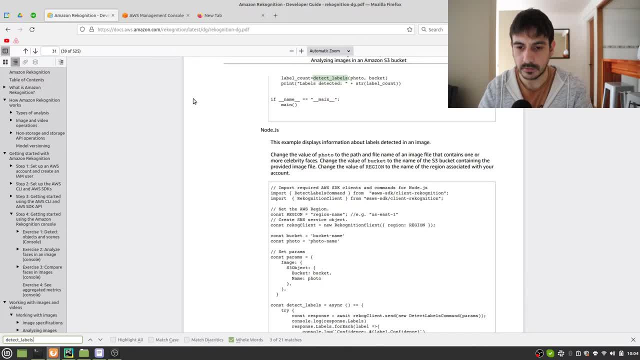 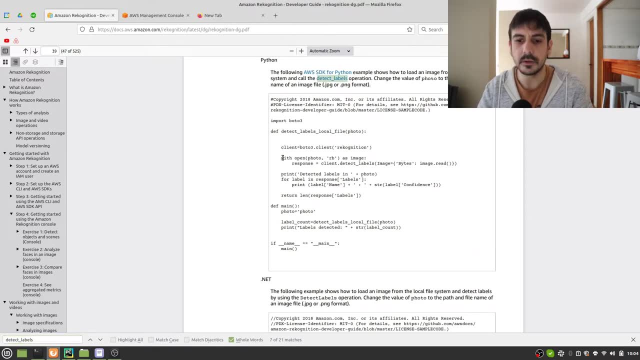 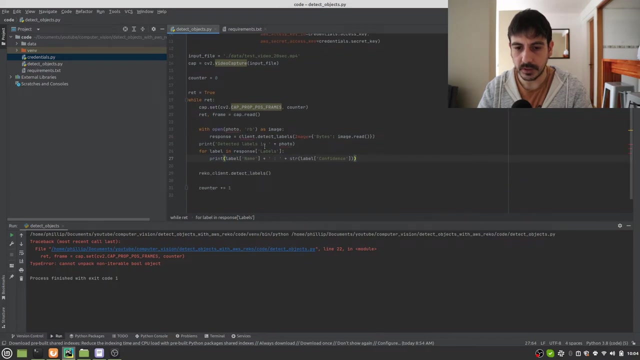 which is the function we are going to use. and if i go down to the python section here, this is how we are going to give amazon recognition, or frame. i'm just going to copy paste this section, okay, now. yeah, that's pretty much it. in order to um to execute this code, i need to save. 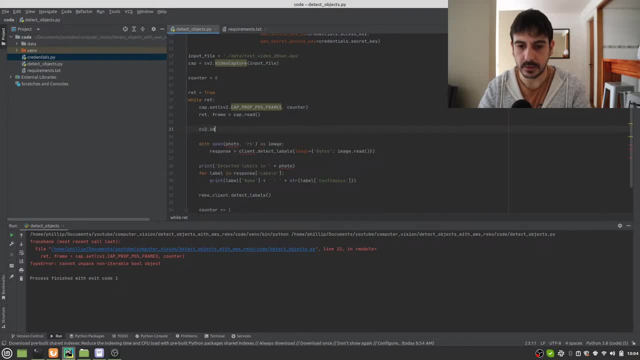 an image. so i'm going to do something like this. i'm going to save my frame in the file name, which is something like this: okay, so this is where i'm going to save my this. just attempt a file name so i can save my video. sorry, my frame, so i can input here. 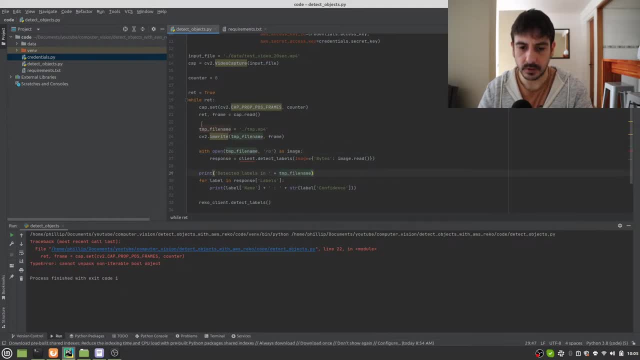 and here, and i'm most probably going to delete some things, but for now let's just remove all the errors. and then i have to delete this auxiliary image i have saved. so it's UsRemove and then temp find it okay. So I'm saving the image in this file name only to have my image available so I can input it into this function, into LVS record. 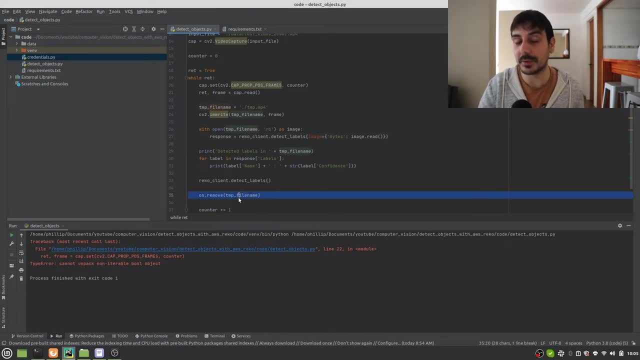 And once I have done all the process, I'm just going to remove this image, because it was an auxiliary image. Okay, so I'm detecting the labels and here I am just printing this. Something I'm going to do only to test if this works properly is to iterate it only for to execute it, only for one iteration. 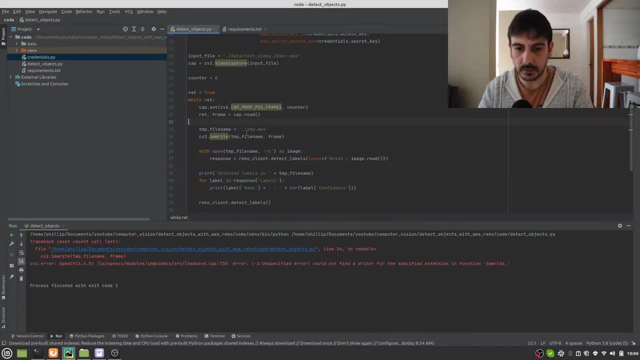 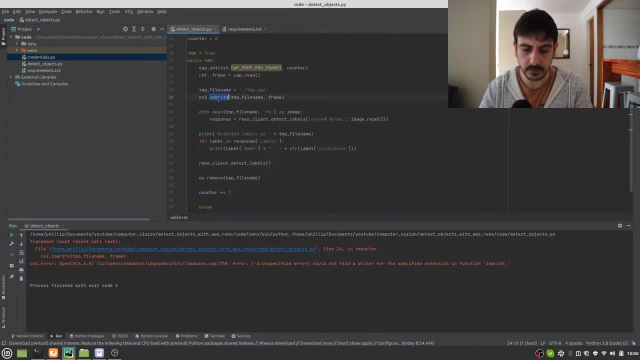 Let's see if this works properly. I have made a mistake in write. I don't see what's the mistake. Then file name, which is fine. Maybe it was not fine. Writer for the specific instruction: CB2 in write. Oh sorry. 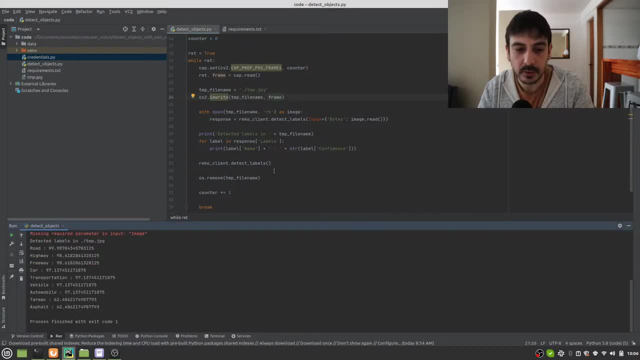 This was not mp4. This was jpg. Okay, so I'm executing this code and it seems it's working, because I am detecting all the different objects And you can see, these are all the objects which were detected with LVS record in the first frame, which is road, highway, freeway, car transportation, vehicle, automobile and so on. 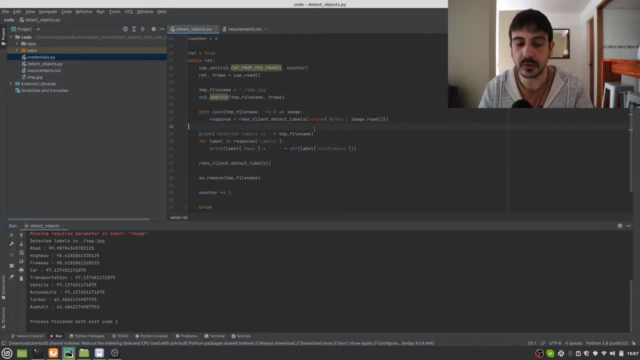 But I'm going to do it again. So I'm going to do it again, But from all of these objects. for some of these objects, we have a bounding box with the exact location of this object, And for other objects it's just like the. we don't really have a bounding box. 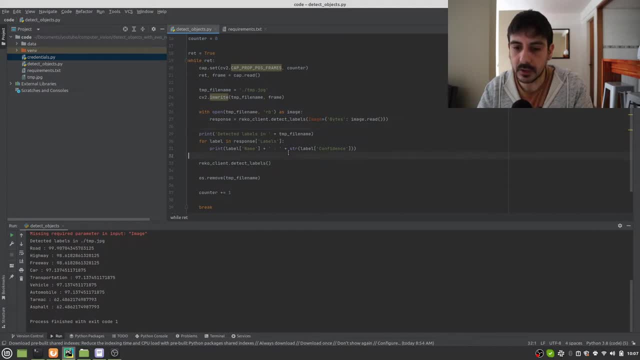 So we want to get only the objects which contain a bounding box. So, in order to make it a little more clear, I'm going to remove this and I'm going to print label And I'm also going to remove this And let's see exactly the object which is returned by AWS. 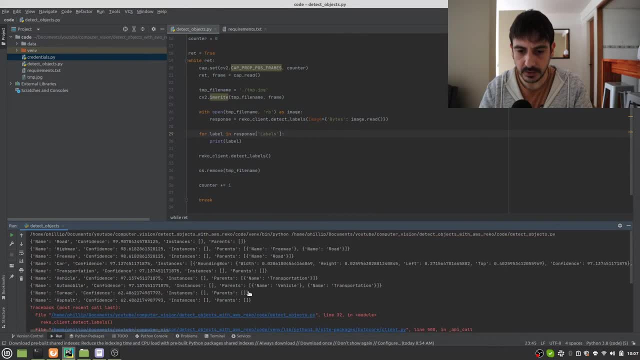 Okay, Let's see I had another mistake. Take label. Oh, I didn't realize, Okay. And so I'm just taking a look at this And you can see that it's not working. And you can see that for some of these objects, or at least for one of them, if I'm not mistaken. 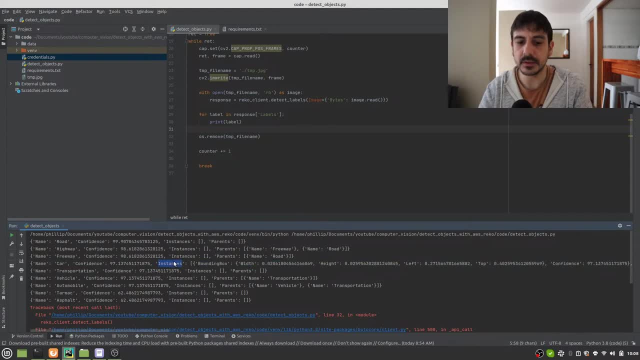 we have this value, which is instances, which is a list, And in this case it's not empty. This is the only case which contains objects. So what I'm going to do is that, for label, in response, labels if label instance. 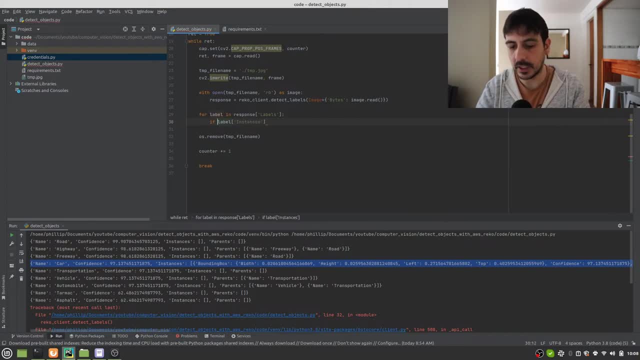 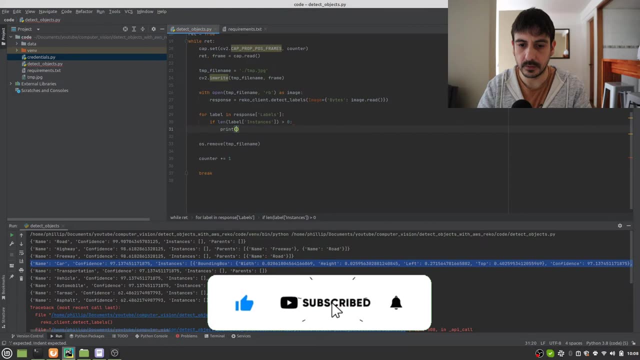 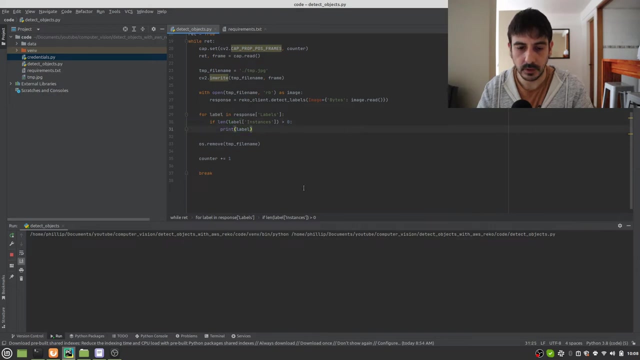 instances, if the length of this list is greater than zero, then print label. Let's see if it works. Okay, Now we are only printing cars. So from all the different objects, Amazon recognition detected in our image, it seems the cars are the only ones that it's. 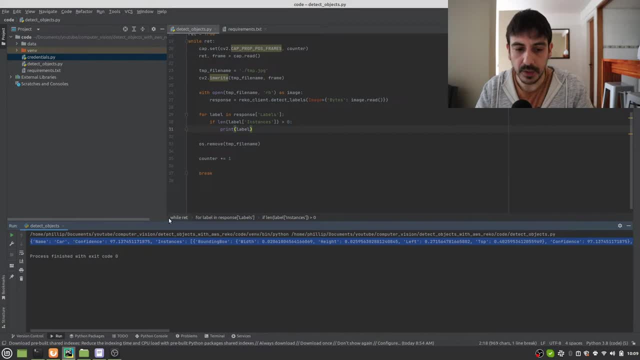 providing us with a bonding box. So what I'm going to do now is to extract all, the all, the all the objects and extract all the bonding boxes. So I am going to do something like, uh, for instance, in label instances, and I'm going to get the bonding box. 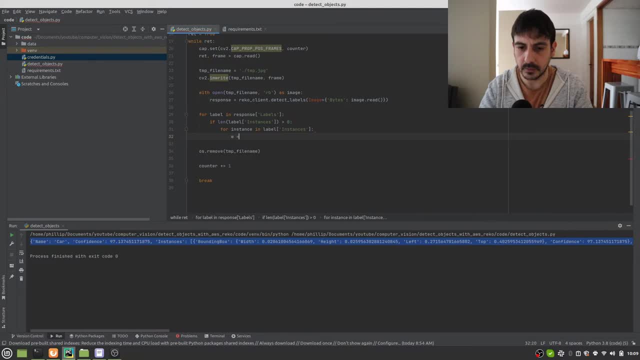 So the width is It's going to be instance, bonding box with, then the hate is going to be the same, but hate then left on top- Oh sorry, This is age. then to extract left, And then the left is what I usually call X and top is what I usually call Y. 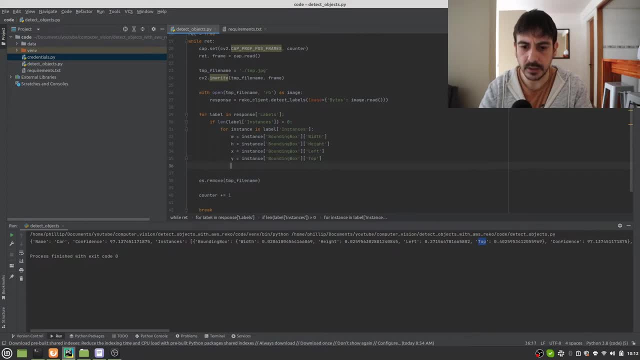 So I have created, I have extracted these four values and let's see if these work properly. I'm going to print these values for each one of my instances and let's see if it works. Okay, It works. now Let's also. 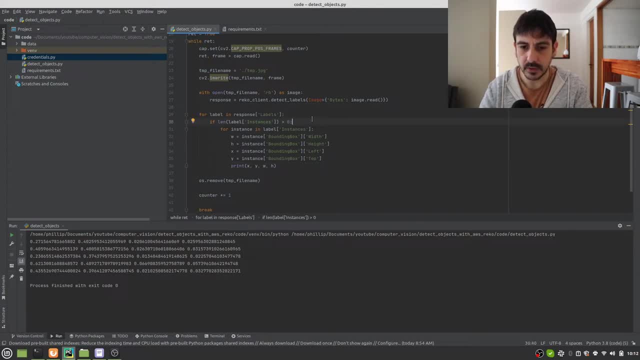 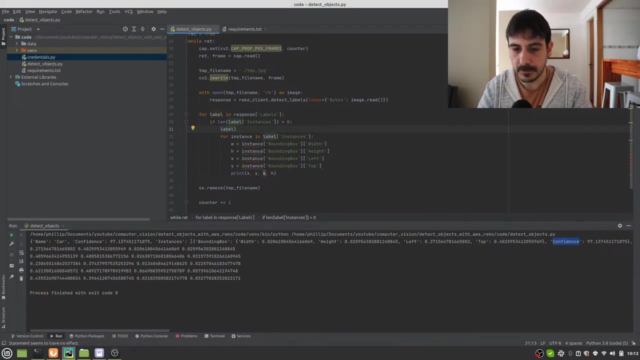 Print. uh, what's the additional information we need to extract? The additional information we need to extract is the object name and also the object confidence. So I am going to do something like um name. it's equal to label name. Something very noisy is going on in my building right now. 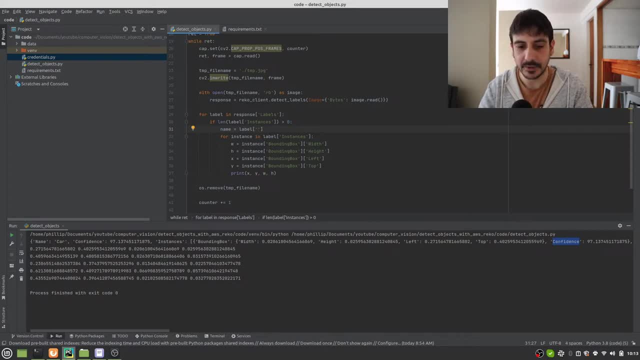 I don't know if you can hear it, but anyway, if You can, then my apologies. Uh, so this is the object name and then the confidence value, which is we are going to have a confidence value for every uh object we detect. 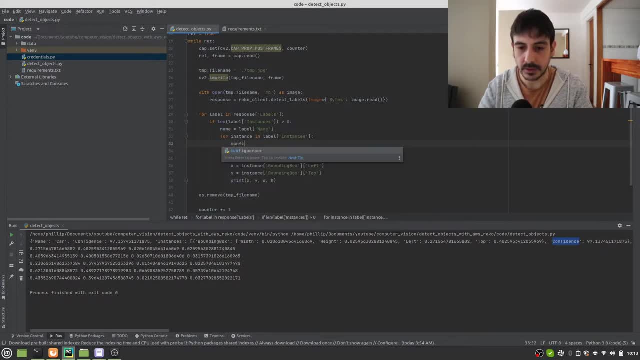 So we need to say something like: confidence is equal to instance. This depends on the bonding box. No, this is only instance confidence. And now let's print everything. So print confidence. let's just call it conf- It's going to be shorter- and then print name. 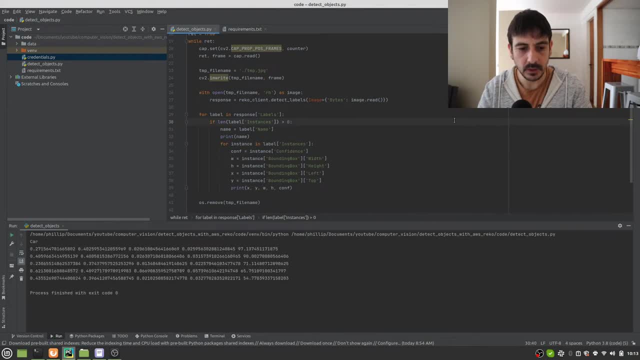 Let's see if everything is okay. Okay, Everything seems to be okay. Uh, the confidence value, I'm going to edit as a value from zero to one, because that's What the that's how the confidence is usually expressed. So I'm going to do something like this: 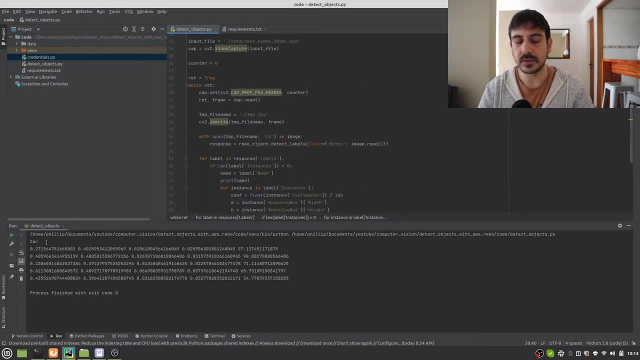 And then what I'm going to do. now we have cars and, as we read, more frames, we are going to have more objects. So what I am going to do is to create a list which is class names, which is going to contain all my classes. 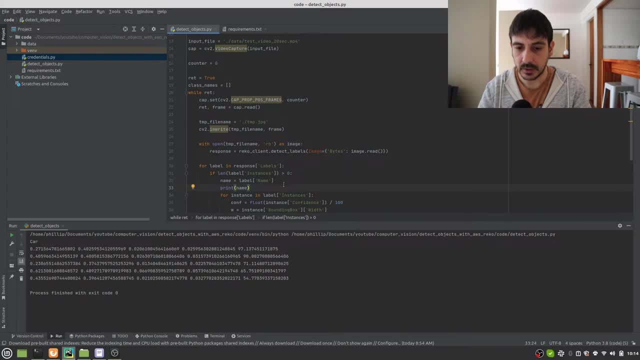 And this is going to be something like: uh, if Name not in class names, then class names, append name. Also, reason why we are doing this is that, uh, we are going to extract all the uh bonding boxes from these images, from these frames. 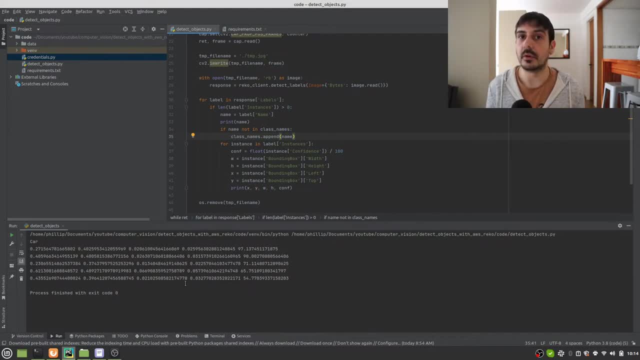 And we are going to save these bonding boxes, We're going to save all these annotations and the way I'm going to save them is using the Yolo format, And it's going to be super Convenient to have our instances, uh names, to to have our class names and also to have indexes for our classes. 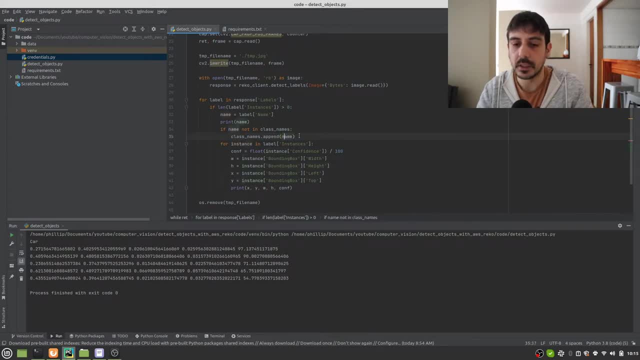 Anyway, this is going to be super convenient and you're going to see why in a few minutes. So I am not going, I'm not going to print the name anymore, because I don't need it. Um, this is pretty much all. 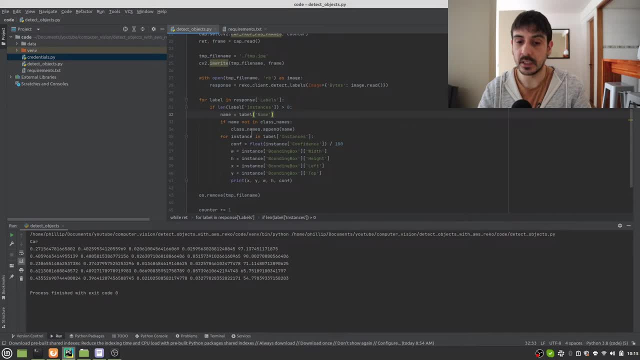 Yeah, this is pretty much how we can extract the class name, how we can save this name and how we can extract the bonding Box. What I'm going to do now is to save all these annotations in a directory which I'm going to call annotations for these. 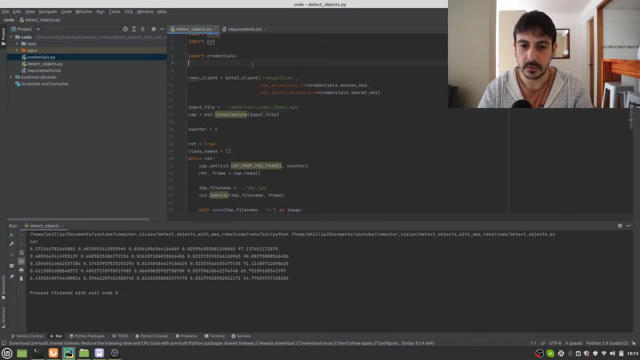 I'm going to greet, uh, an output directory which is going to be something like output beer. I'm going to say it's here output. Then I'm going to have my aunt's deer, which is going to be Something like: I'll put the your aunts, and then I'm going to have my image, this directory which is going to be here, because not only I'm going to save my annotations but I am also going to say my images. 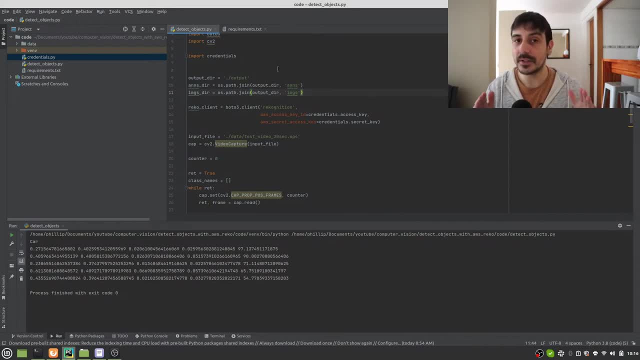 I am going to take this as an opportunity to create a very small data set of images and annotations. So I am going to extract the annotations with WBS record, But I am also Going to save the images. I am going to save the frames in another directory and I am going to follow the Yolo format in order to do it. 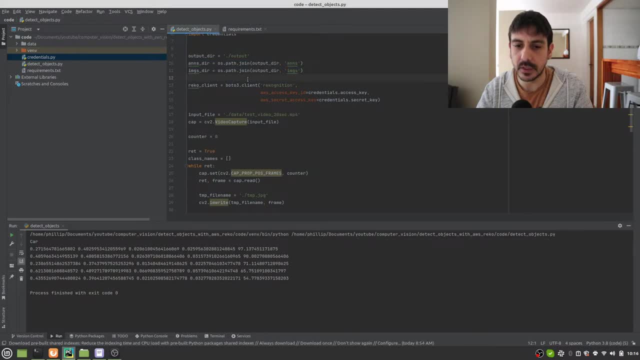 So, um, once I have created these two directories, I need to save the annotations, and I have one rotation for each frame, So this is where I have to do it: If red, if I have a new frame, then all of these. 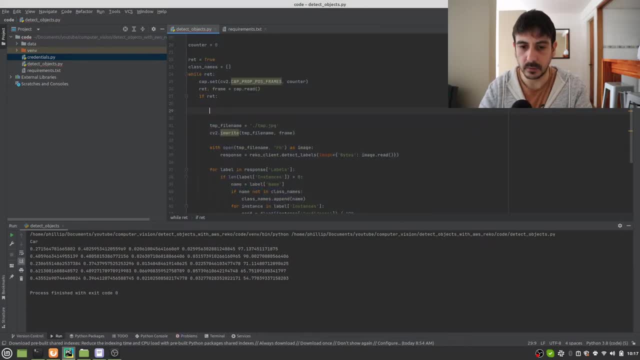 And also with: I'm going to do it like this and file open, um, something like us, but join and steer, And then this is going to be: oh, oh, dot, TXT, dot format, Um, basically, Yeah, Yeah. 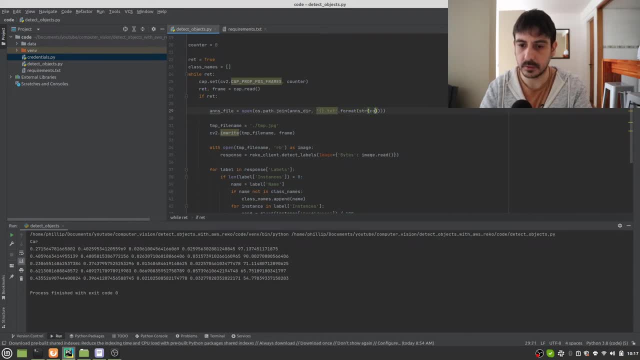 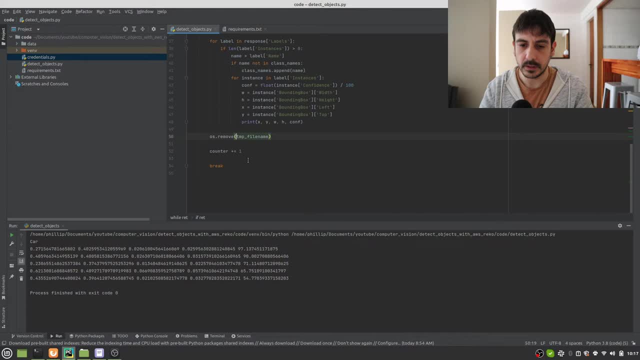 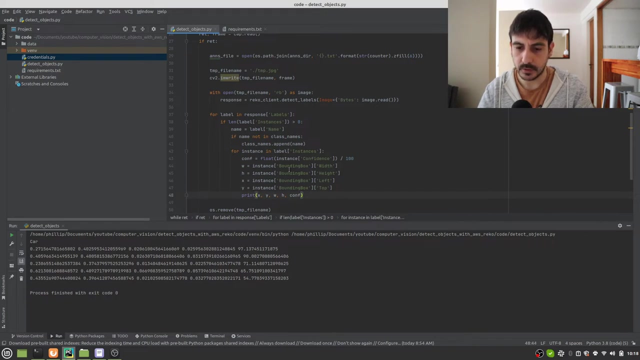 I think it is, And then I'm going to close these file around here, but close, I'm going to make it nice and let's make the incremental at the end, okay, so what I need to do now is to print these values. this is going to be in yellow format, so what I'm going to do 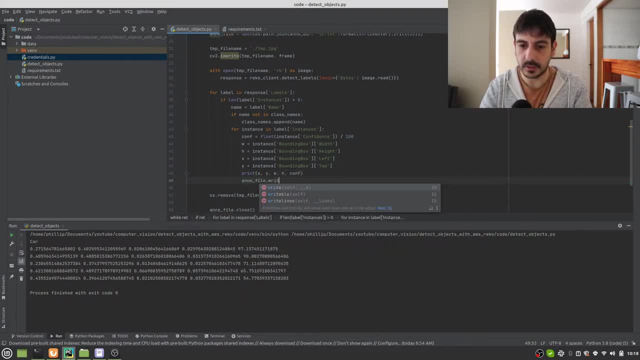 is ans file dot write. this needs to be in yellow format. so the first element is the- let's write a yellow format here, only to remember which is class index. then is X, C and Y C, which are the positions of the center of our banding box. this is not the upper left corner, but this is the center of our banding. 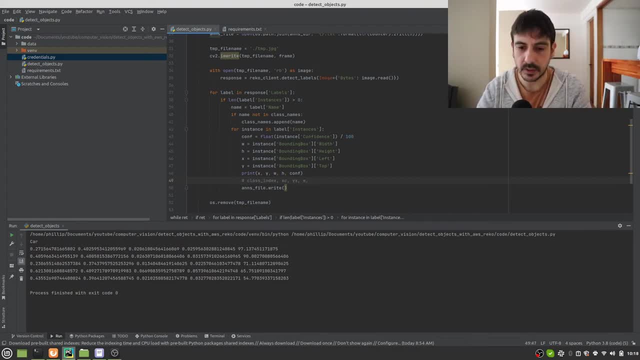 box and then or with a height, okay, and this is going to be like a yellow modified version which is going to contain also the confidence, because if we are saving our annotations in yellow, the annotations are only these values, right? I mean, when we are not 18 objects, we don't have a confidence value, because 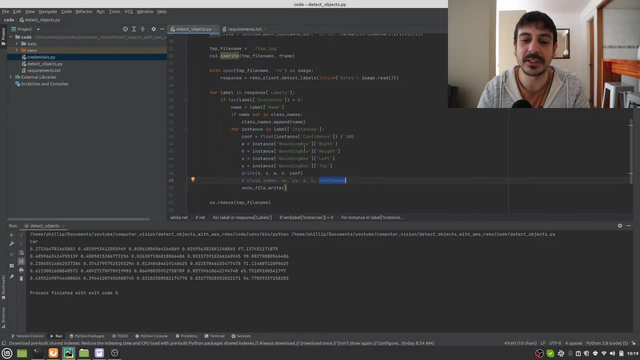 those are rotations, but in this case we do have an addition. so because these annotations come from an object detector, so I'm going to save the confidence value too. so we have one, two, three, four, five, eight, six values which I'm going to save. so I'm going to do something like this one. 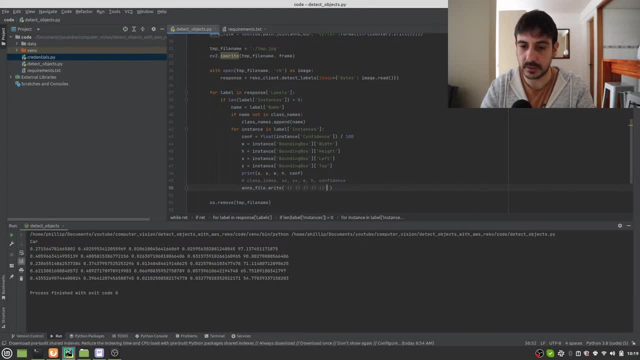 two, three, four, five and six and new line. ok, and now this is going to be format: class index, which is going to be class name, that index and then my name, right? so this is why I'm doing this, because here, in this part, what I need is an index. I need an interval value. 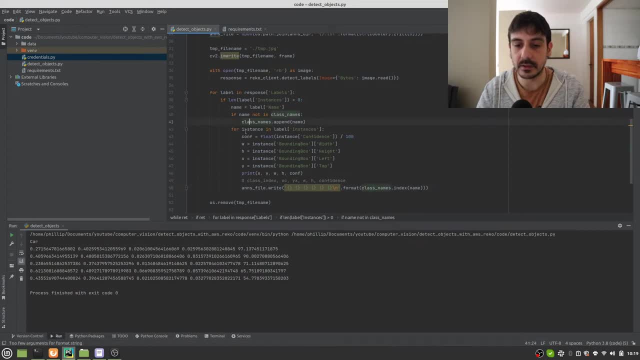 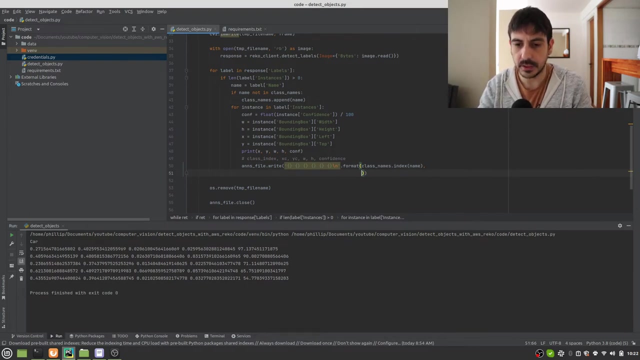 and the way I get this integer value is by taking a look at what's its index in the class names list. so this is going to be enough. then the XC and the YC values. these are going to be something like my X value plus W divided by 2. right this: 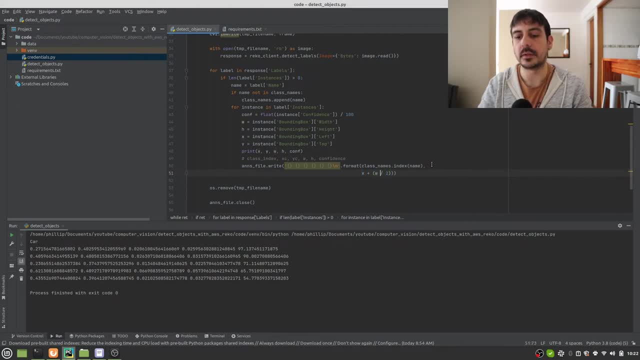 is my upper left corner. so if I add this value I'm going to get the center of my bounding box. then this is going to be exactly the same, but for the height and Y, and then I only need to save W and H and my confidence. so everything seems to. 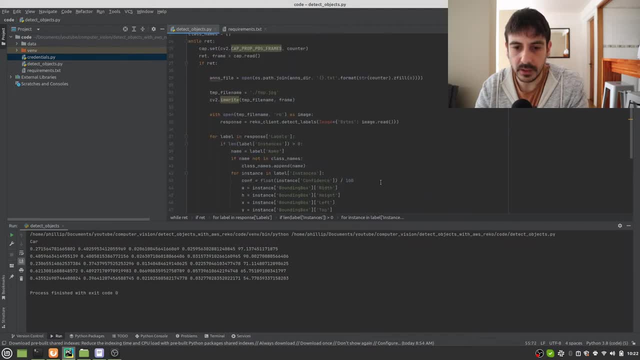 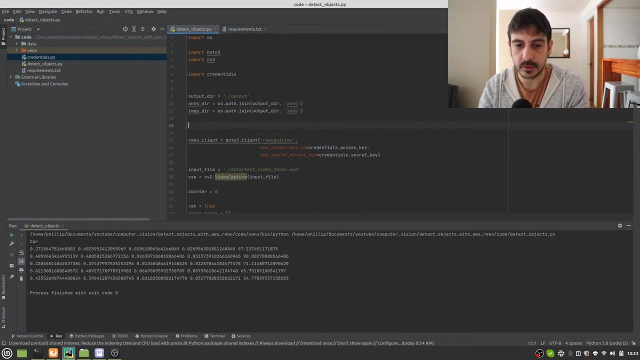 be ready, and something I haven't done is to create this directory, so otherwise I'm going to have a huge error. so for dir in output dir and dir and images dir, if osPath exists dir, then I need another library which is shutil, then shutilremoveDir. 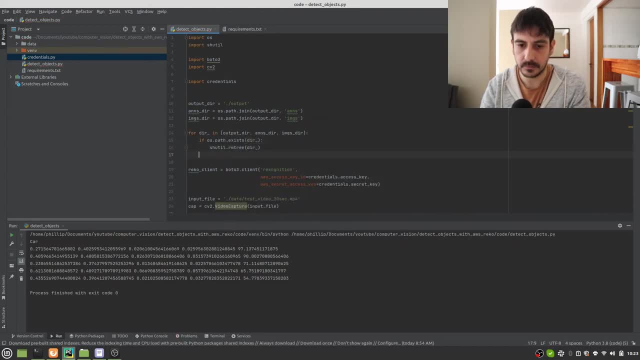 then shutilremoveDir and then I know for sure the directory has been removed, so it's made it dir. okay. so this is because every time we execute this code, in case we have a previous execution, in case we have annotations from a previous execution, we just want to delete everything and to overwrite or detections. 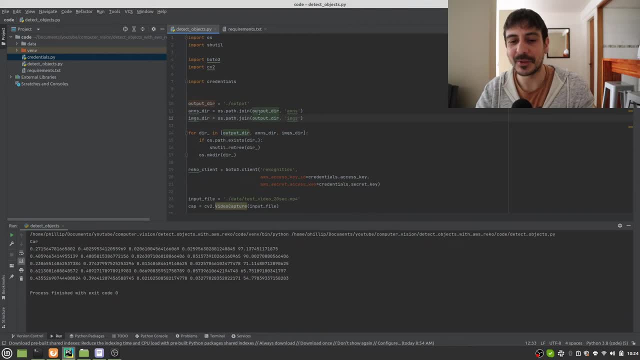 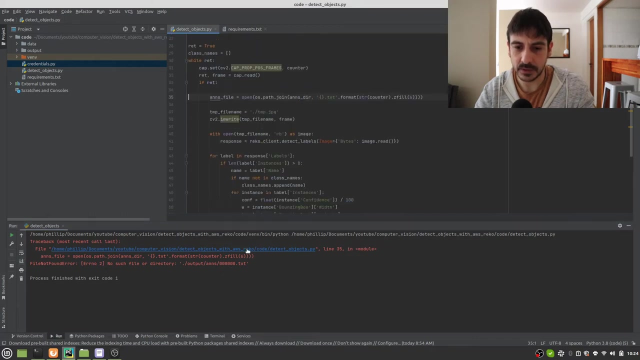 or annotations. this is what we want to do in this specific case. i'm not saying this is a good practice always, but anyway, this is what we are going to do now and let's see if this works. obviously it doesn't not. such file or directory- this is here ans directory. it should exist. why it say it doesn't? 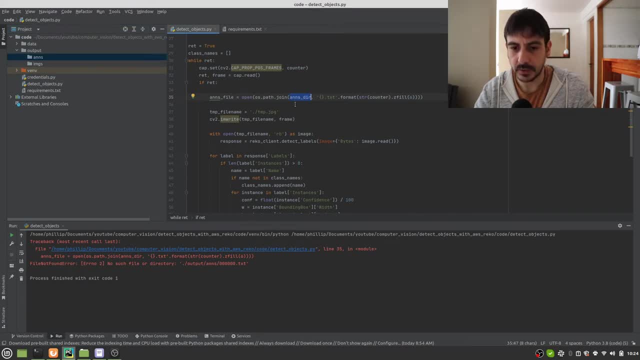 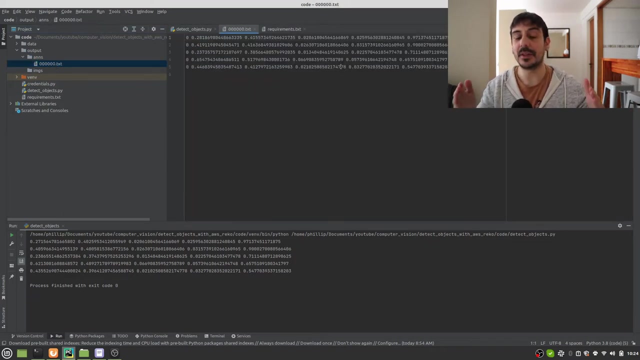 and ah, because i have opened this file but i haven't specify how great. okay, let's see now. everything seems to be okay and if i take a look at here, i have my annotations, so everything is pretty much ready. now we are at a 95 completion. 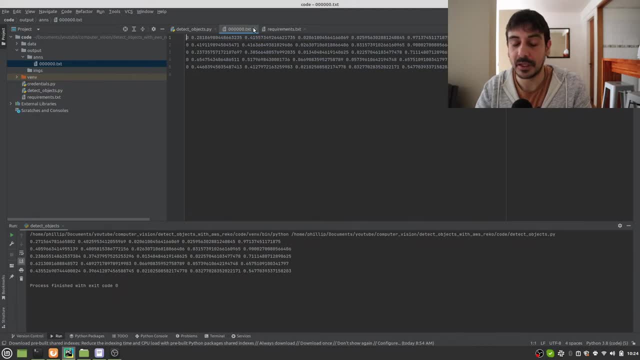 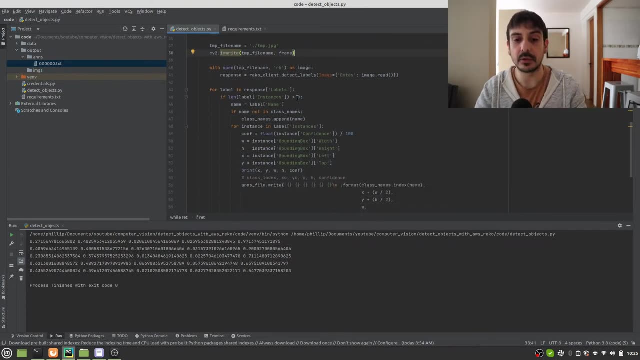 so everything is pretty much ready. now we are at a 95 completion. everything seems to be okay and if i take a look at here, i have my annotations. Now we only need to do a few edits, a few more things. So now we have saved our annotations, but we also need to save our images, because I 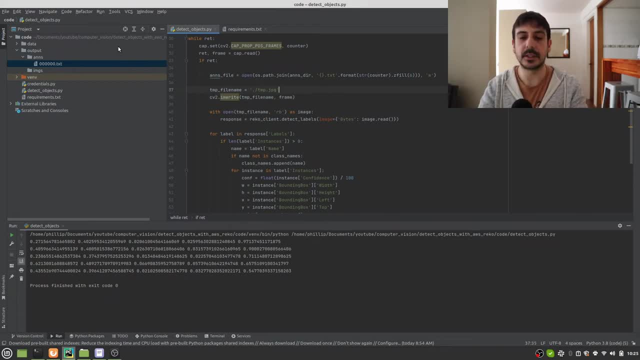 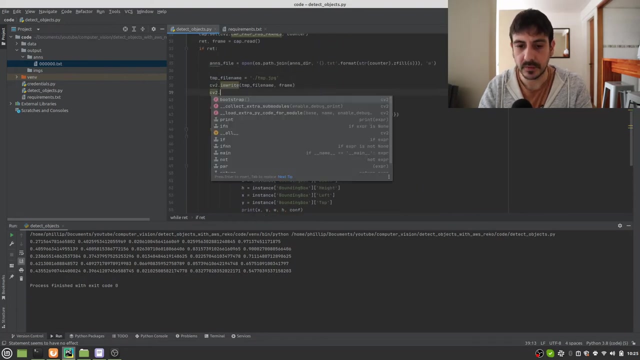 mentioned that we are going to save like the entire dataset of frames and annotations, So what I am going to do is to save it here after I have saved this temp image. I don't need the temp image anymore, but I'm just going to save it anyway. 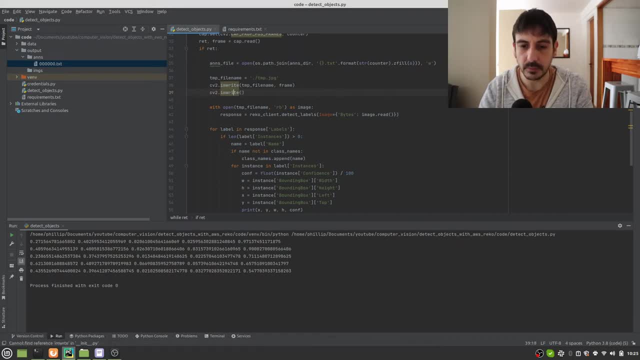 I'm going to do cv2 in write. I mean, what I mean is that I don't need this, because if I am going to save the image here, I could be using this same image I'm saving here to give it to the record. but I'm just 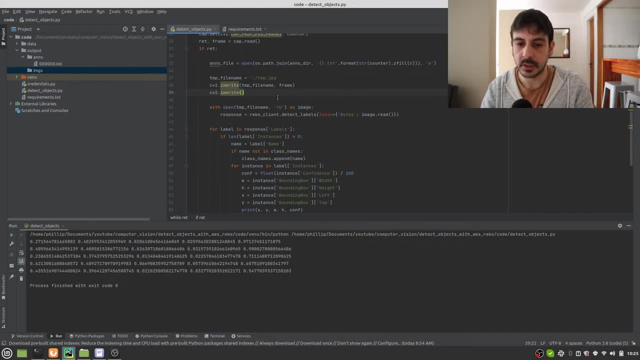 going to keep writing this temp image, So cv2 in write. This is going to be super similar. This is, but now, instead of the dot txt, I am going to save it dot jpg. Okay, So that's going to be all and I need to give it frame. 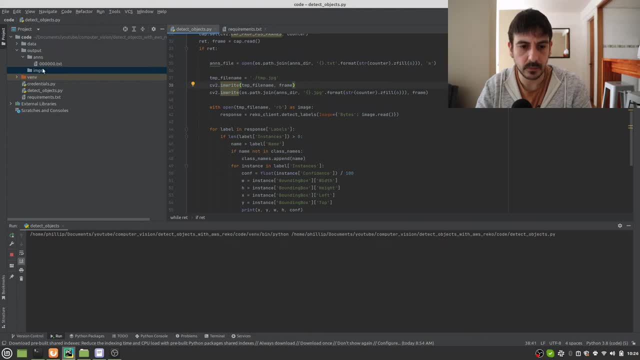 Let's see if this works. If it works, I should have an object. Wow, I don't see It. sometimes it takes some time to refresh and it's not the case. Oh, I have saved it in the same directory, so I need to change it to images there. 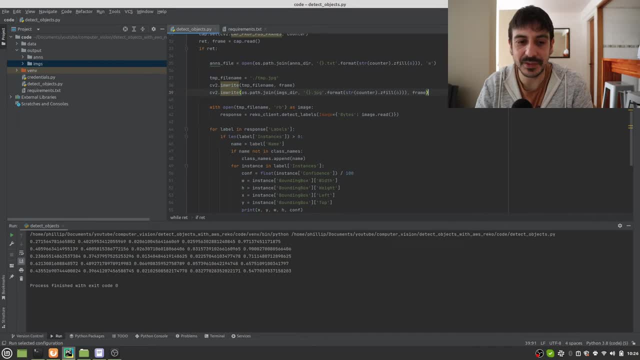 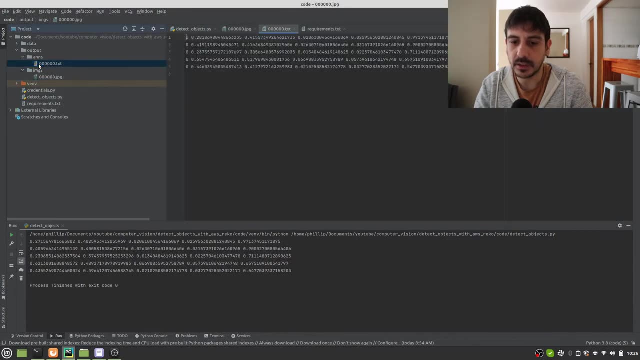 This is why it's important to test your code at every single time. So this is it. Now I have my, my initial frame and my initial annotations for this frame. So what I have to do now Is Just continue this process for all my frames, right. 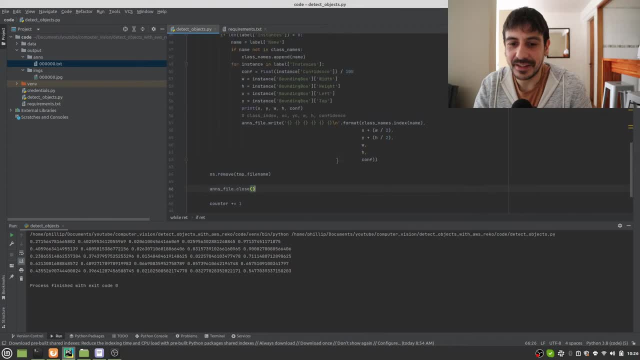 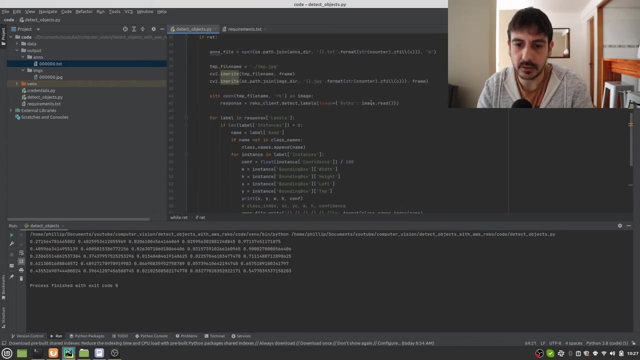 Yeah, I have absolutely done everything. Uh, the only thing I'm going to do is to plot some of these annotations so you can take a look at how they look like. So, um, this is not really needed, but in order to show you that everything 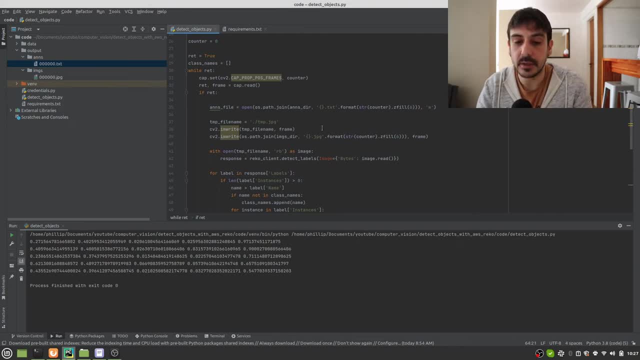 is working properly and that we are in fact detecting everything we need to detect. or I mean, in order to show you what are the detections we are getting from AWS RECO, I am going to do something like this. Um, I'm going to do CV2 rectangle. 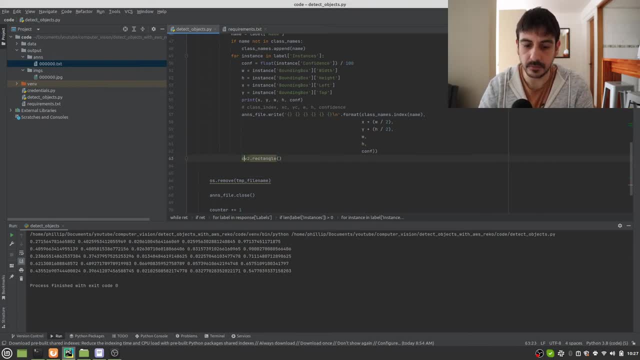 Tangle. I'm going to draw a rectangle in each one of these frames. Frame: Yeah, After I saved the frame, I don't use it anymore, so I can just draw things on top, Is? It doesn't matter? This is going to be frame. then two values, which are going to be the upper left. 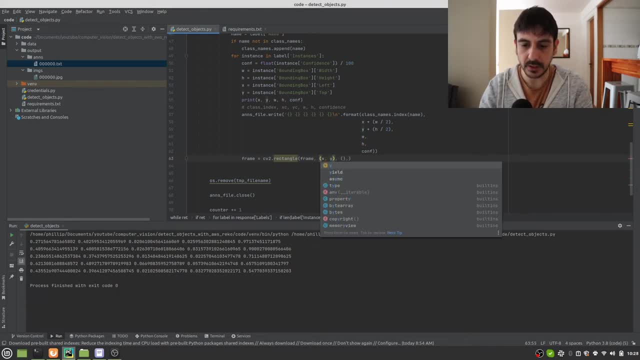 This is X and Y. I need to make this an integer, because now it's a relative value, but I need to give it, like the, the, the, the actual value, then an integer with the X- Y position, And then this is going to be X plus W, Y plus. 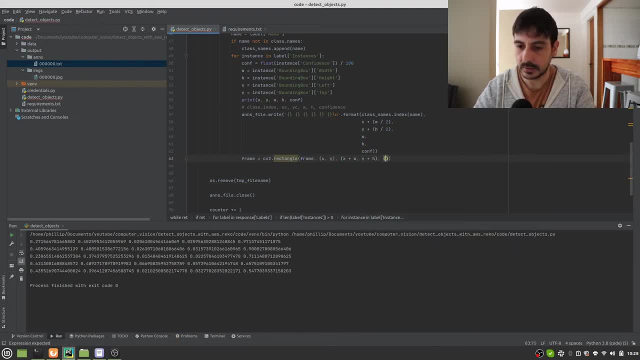 Double, uh hate. Okay, So this is going to be, um, a color which I'm going to choose: green. Um, then the width value, which I'm going to make it three. Now, what I'm going to do is to create a new values. 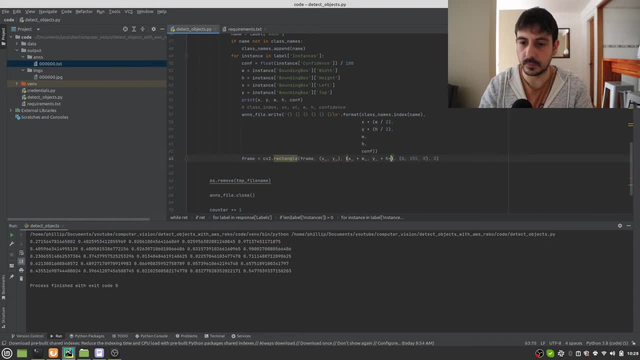 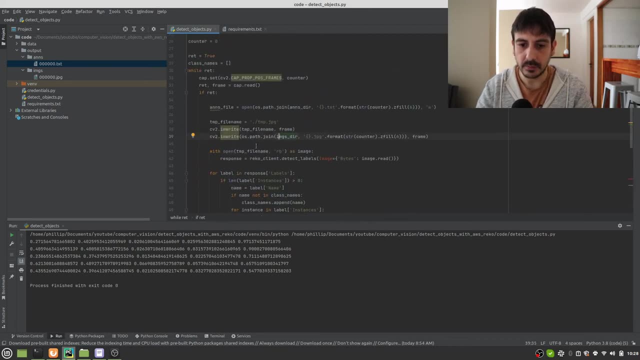 So I can just define these new values, Okay, And I also want to need the width and height of my image, So I'm going to do something like capital H, capital W and nothing, And uh and uh, this uh character uh, which I'm not going to do. 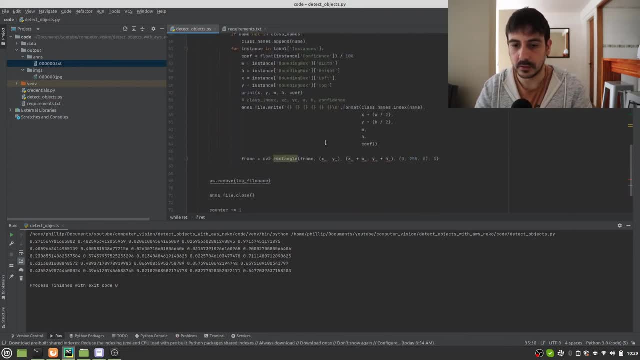 So it doesn't matter, It's going to be framed that shape, Okay, And now X C, sorry, X, uh, and this character. it's going to be equal to Integer X times my big W. yes, this is going to eat. 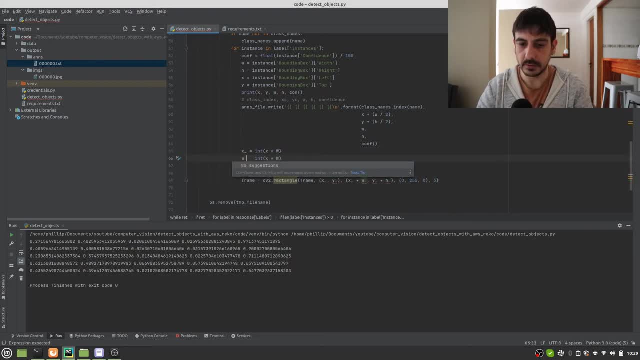 Then I'm just going to copy and paste: my W is going to be these, um, my wife is going to be these, and then hate is going to be this. This is going to work, I think, Okay, Okay, I think, let's see. uh, this is going to be my frame. 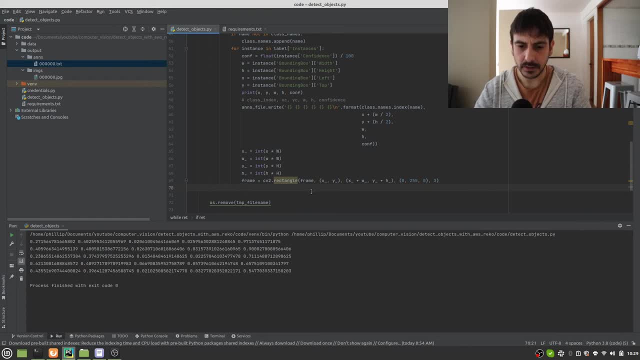 So I'm going to draw all the bonding boxes and then I will need to plot this frame. Yes, I'm going to need to pull it here so I can show you how it looks, how it looks like in show. I haven't imported, but we'll leave. 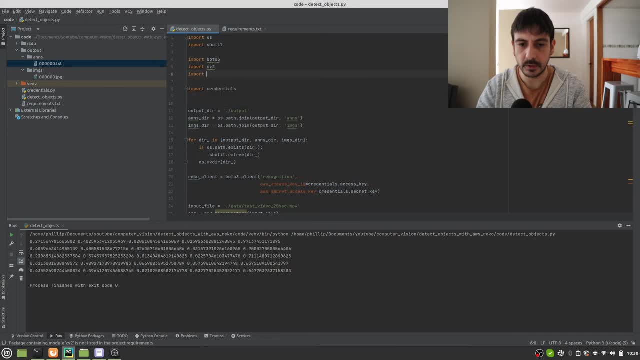 Right, Yeah, Uh, I need to import it. Matplotlib dot piplots As PLT, So PLT dot in show. Uh, this is going to be my frame and that's it. Then Don't show. something you have to do is to convert this frame to, uh, another color space because, um, the way it works is that the frame is red in BGR but Matplotlib needs to be red. 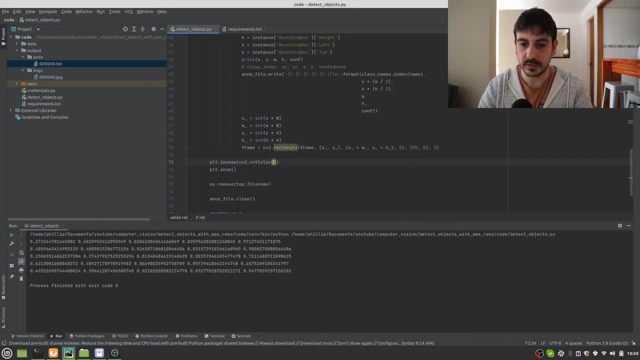 So I'm going to convert this frame to another color space because, um, the way it works is that the frame is red in BGR, but Matplotlib needs to be red. Matplotlib needs to convert it to RGB. So let's do something like this. 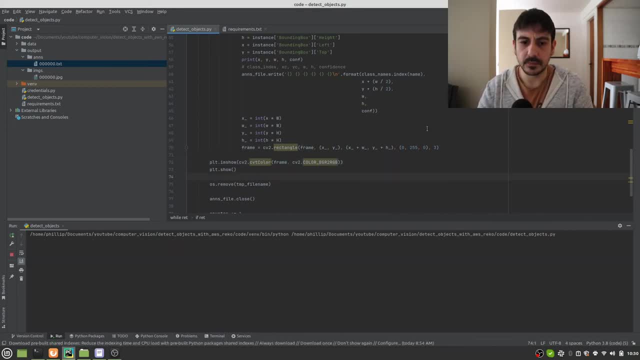 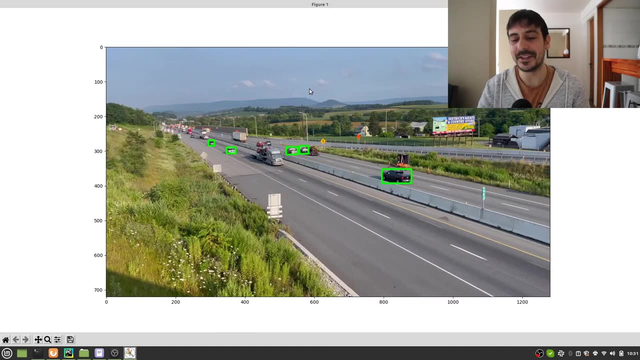 Okay, And that's going to be enough. Okay, Let's see what happens now. We are saving our, our frames on no orientations, but we are also plotting everything And, if you can see, everything is working properly. uh, these are all the objects we are detecting. 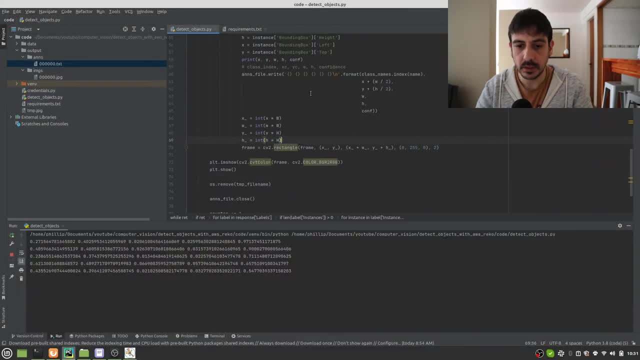 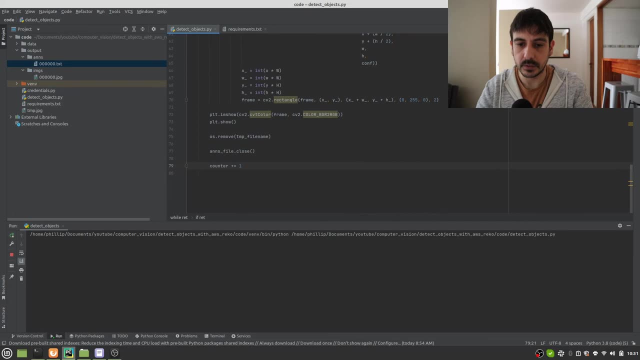 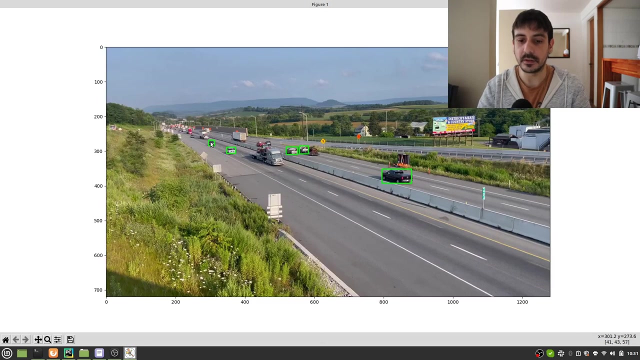 I am going to reduce these with value Um, I am going to Con Uh, execute it for more, More frames. So, in the first case, these are the objects we are detecting in the first frame. These are the- uh, yeah, the cars we are detecting. 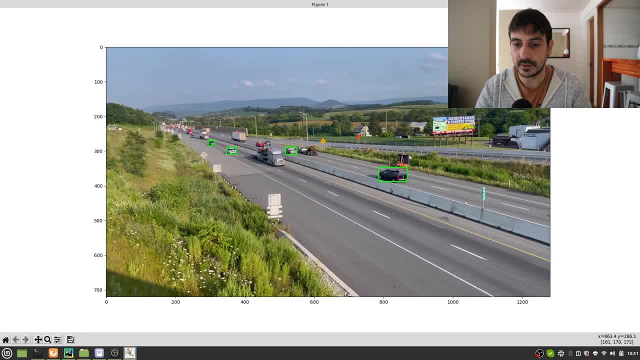 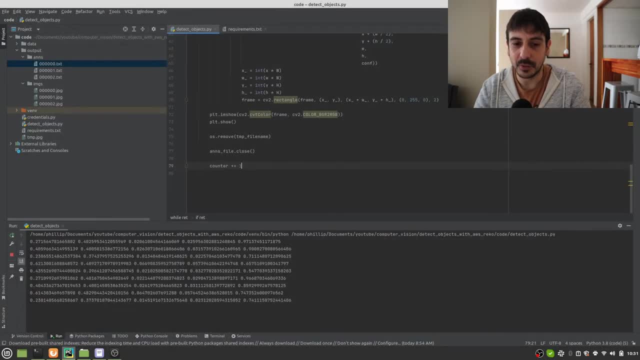 Then, if I continue to the next frames, these are the objects we are detecting, which is, pretty much the same objects, but one frame later, uh, and moving on. So I'm just going to show you two or three frames and that's it. 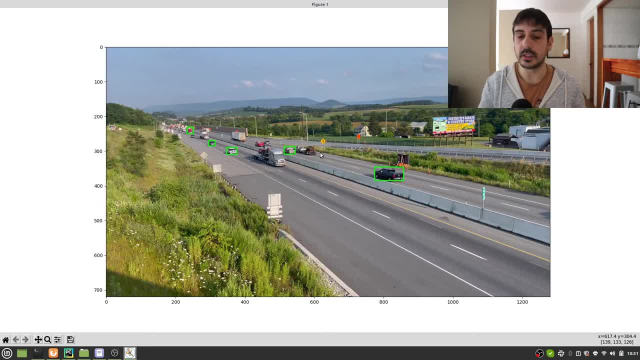 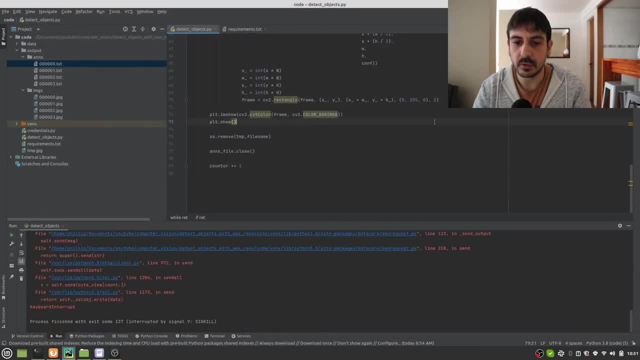 So LDS record is working properly, Because we are getting all the objects, uh, or we are getting many objects from this frame, and or script is working properly as well. Now, this, uh, this plotting was only to show you the bonding boxes. 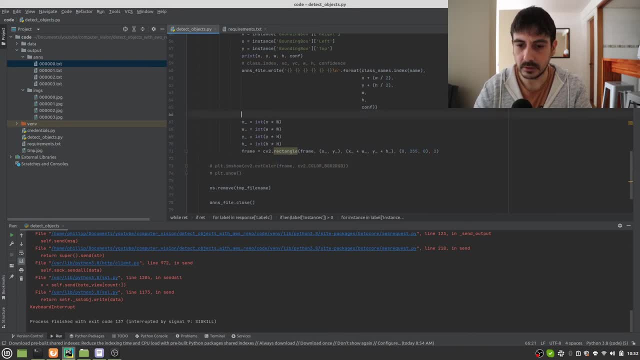 I don't really need them in order to continue. I'm going to comment it just in case I want to get back to it later, And what I'm going to do now is to. I have removed my frame. Uh, my break. 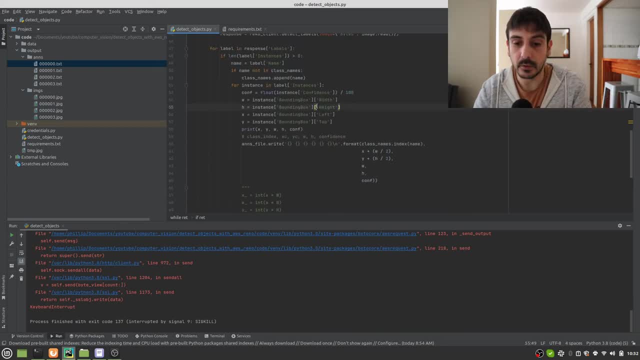 So everything is ready. Yeah, Okay, Now I'm going to execute this code for all of my images, And this is an important step. I'm going to comment this too, because now we see that it works for one image and for a few images, but it doesn't mean that's going to work for all of our images. 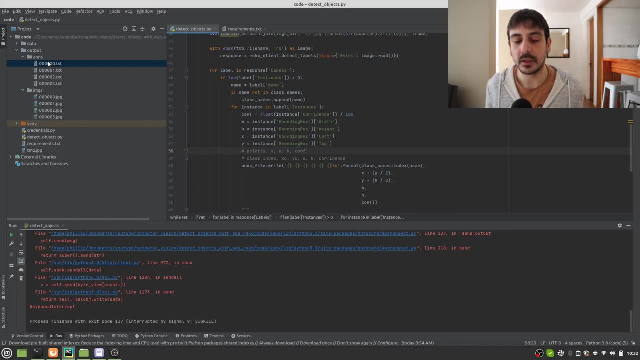 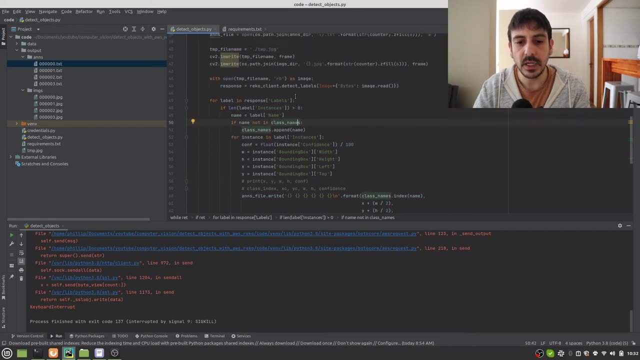 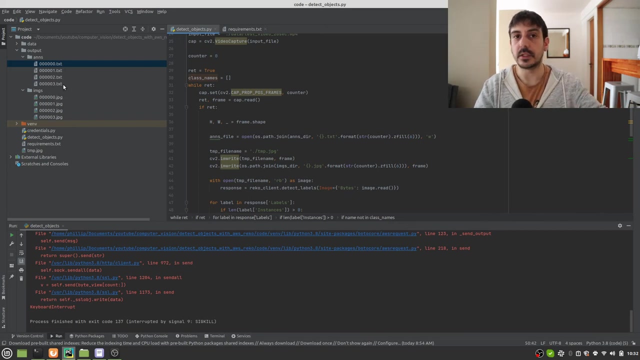 So it's going to be a very good exercise to uh just execute it in all the frames and to see if we catch any other bug or something And something else. I'm going to Uh because he's going to be very important in case I want to use these annotations in a later stage. 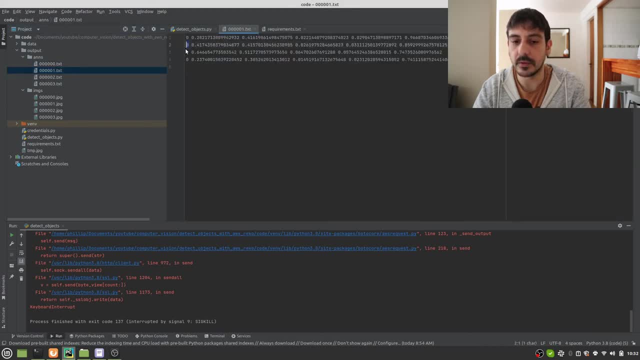 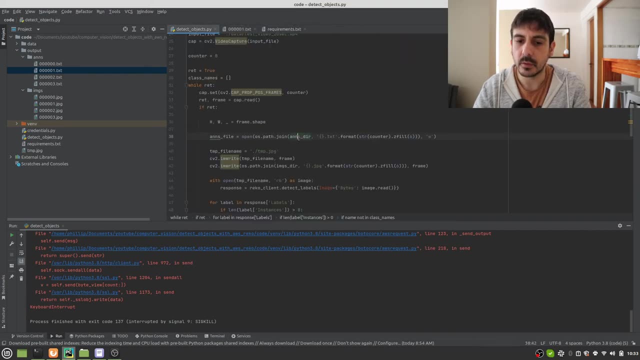 I'm going to, I want to make some sense of these values, right? These, um, these values. I'm saving the class, the class indexes. So what I'm going to do, in order to make it very uh, Yolo compatible, Yolo like, is to save an object which is going to be called class names. 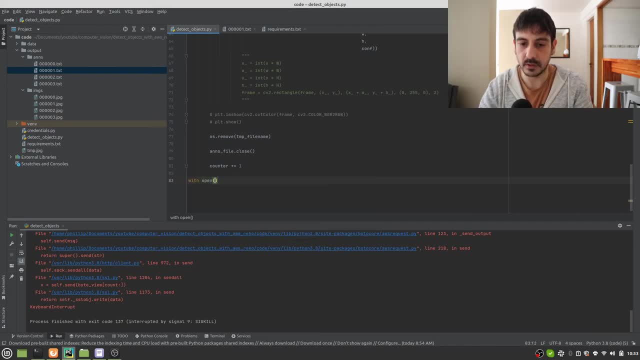 Um, this Is going to be with open, but join output directory and um class dot names. Yes, And this is a w. It's going to be as I've told you. Uh, and I'm only going to write the name. 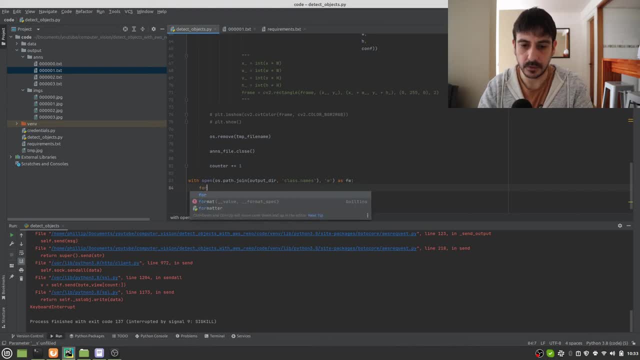 So, uh, for name in class names, this is: uh, I've told you right, Something like this. and um new line, correct Format name. Okay, And I am going to do this and then close. This is going to be enough. 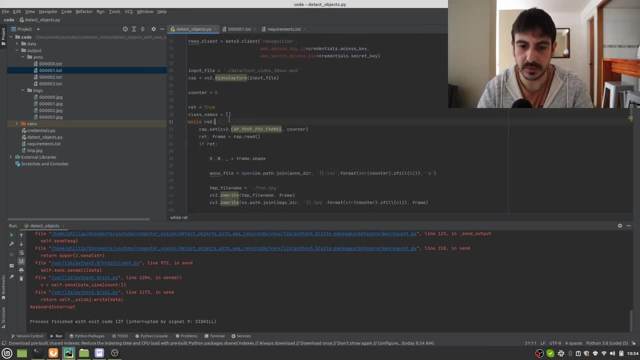 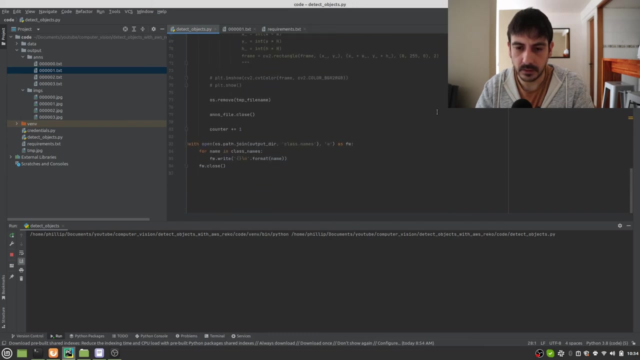 Yes, And I'm going to execute it for 10 frames and to see what happens, while red and counter my ignore lesser than 10.. So let's see what happens. Uh, now I'm not printing anything, So I will not know what happens until this is completed. 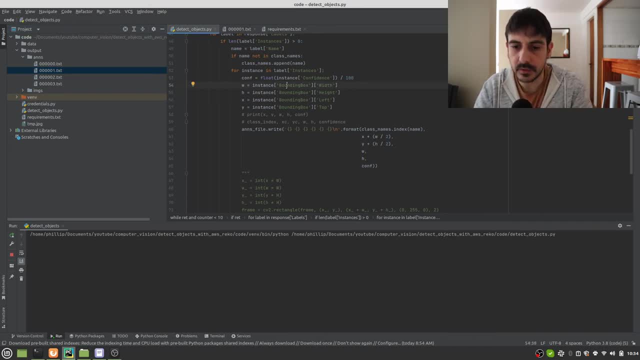 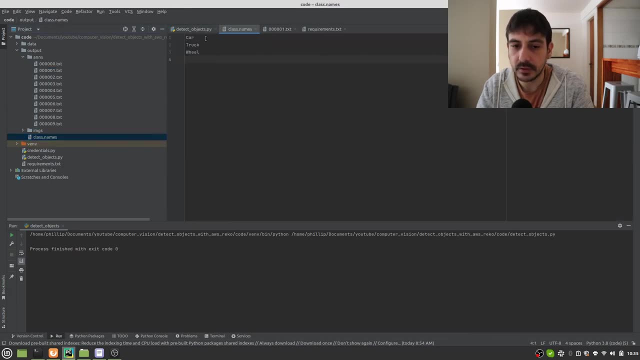 Um, okay, It may take a few seconds, but at the end I should have. okay, it's done. I should have this class names file and these are the uh class names. we have detected car And it seems that in some of the objects we have also detected tracks, because there are a few tracks. 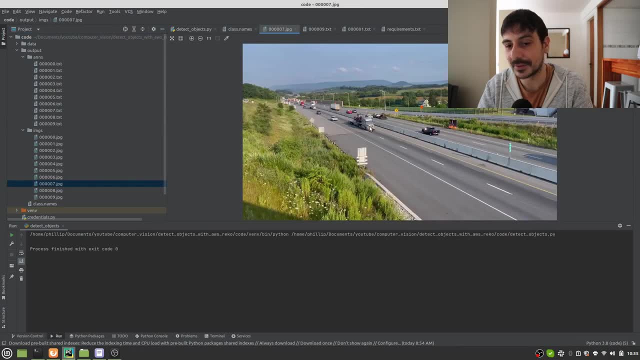 Uh, going on, If I show you this image, we have this track, So it makes sense. We have detected a track and also, it seems, record has detected wheels, which also makes sense because there are many cars and many trucks and many vehicles going on in these highways. 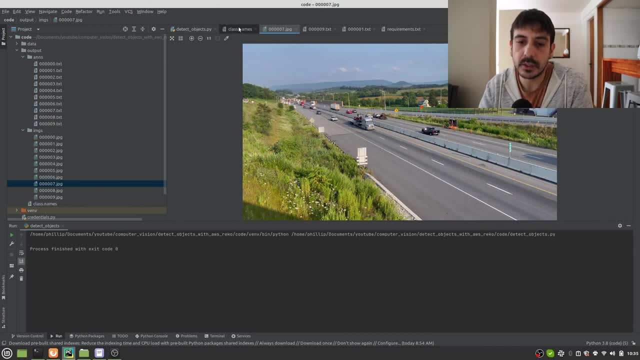 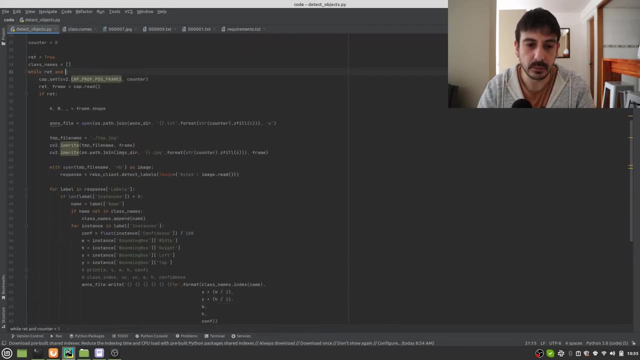 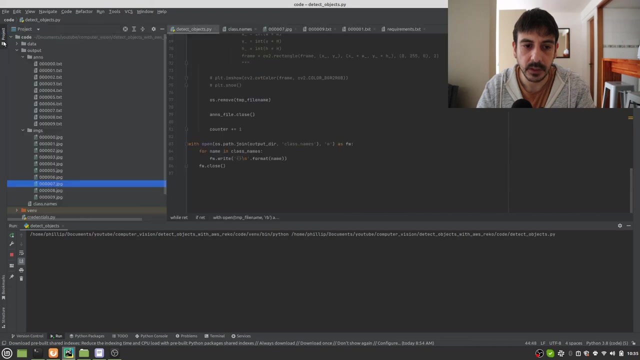 So it makes sense. We have detected wheels as well. So, anyway, this means he's working properly, and now I'm just going to execute it in the entire video. So I'm going to remove these And I just have to wait. um, just in case I have I find any error or any something, I am going to show you the um. I'm going to post the video now and I'm going to fast forward to the moment is completed or the moment this has an error or something. 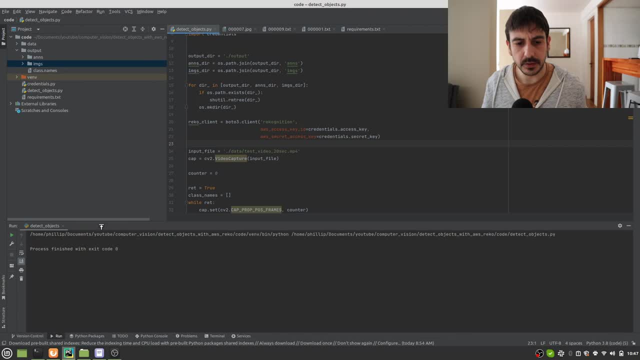 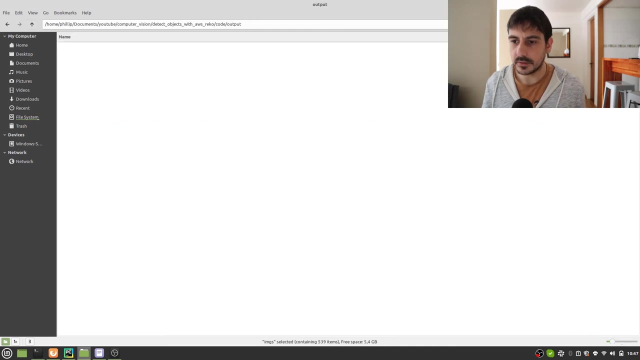 So see you in a few minutes. Okay, So the execution is now completed. if and if I go to my directory, I obviously I had no error or anything, So I assume everything was executed correctly. If I go to my images and ans directory, I see I have 539 items in each one of these directory. 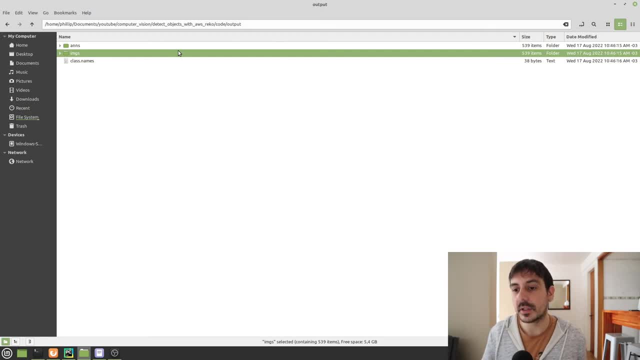 I have the same amount, So that's important And it's around 600.. So it seems it's okay. It seems the input video is not 30 frames per second, So this is pretty much why we are not getting a 600 frames. 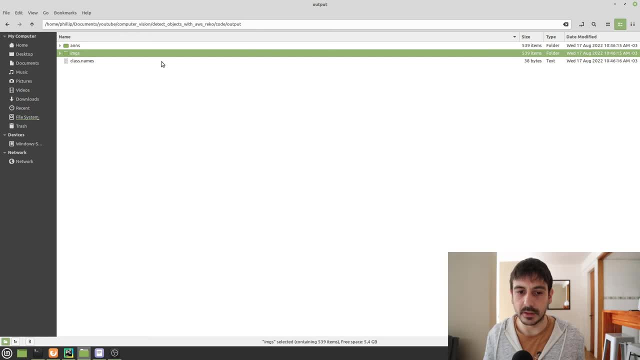 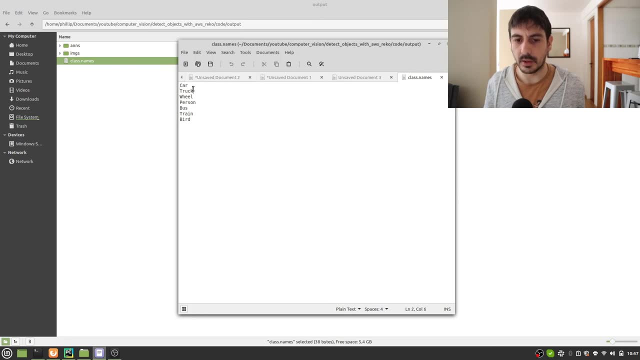 If We took 20 seconds. it seems it's lower than that, but it doesn't matter. And these are all the names, all the classes we have detected through all these frames. We have cars, trucks, wheels, person, bus, uh, train and bird. 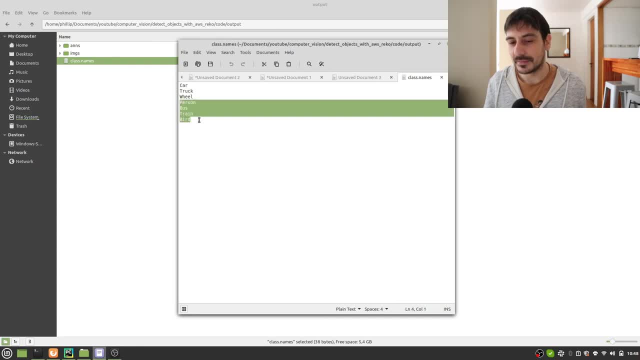 I I'm a little surprised about these uh classes. I watched through the video and I didn't see any train or any person or any more. Maybe there are passes, I don't know, But I'm very confident. there is not any beard. 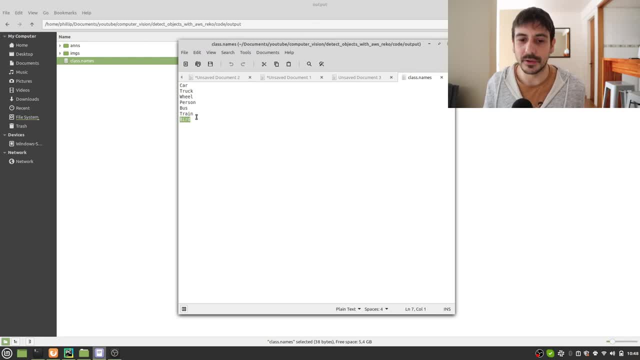 So I don't know. but anyway, maybe these were detected with a very low confidence, or maybe, in fact, there was a beard going on in some moment. I don't know, It doesn't matter. The important thing is that we have completed or object detection using record, and we have also created or very small data set. 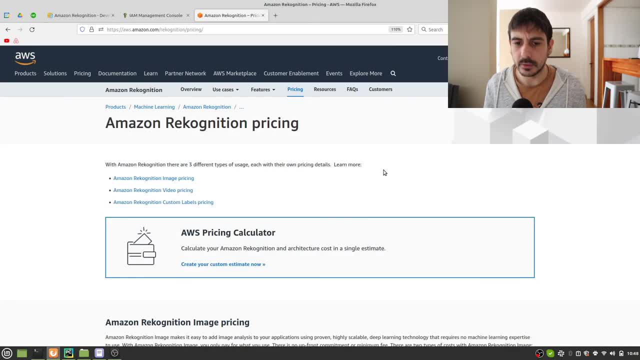 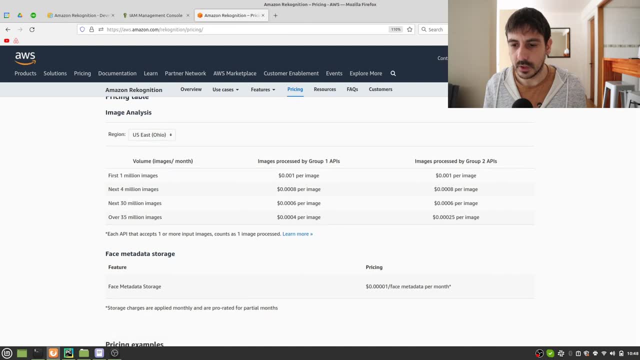 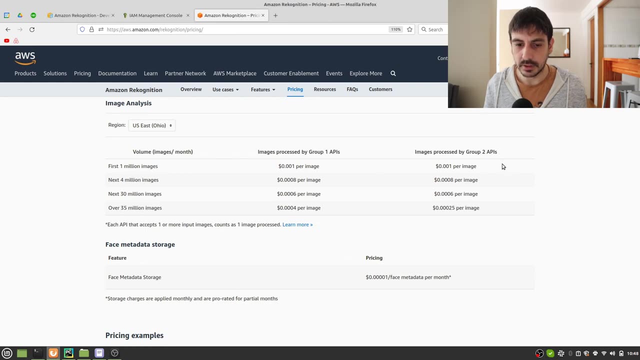 And something I forgot to mention and then I'm going to tell you now, is that the earliest record is a very interesting service, But it is not free. Obviously, you have to pay for the images you are detecting, but the good thing is that it's very, very cheap, or I find it very cheap. 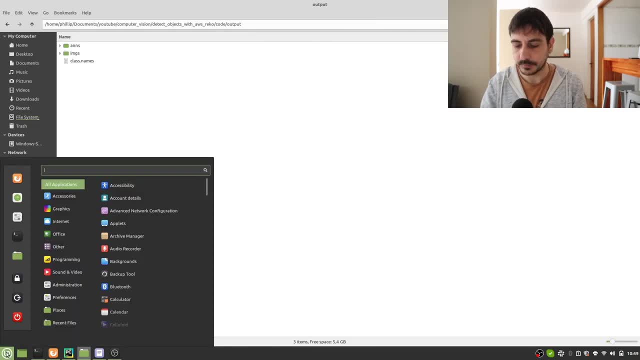 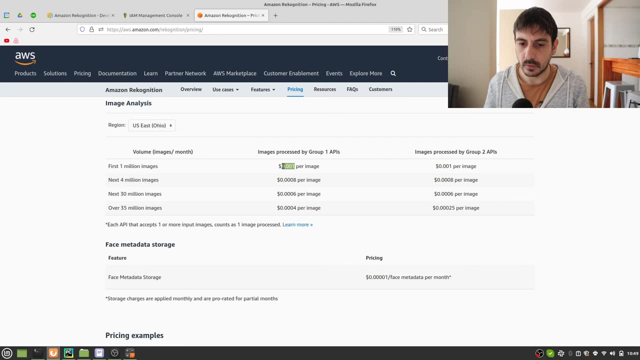 In our case, we have detected 539 images and at a price of 0.001 per image, It means we are going to spend 50.. Uh, four cents in this entire process, which is not really a lot. So it's very cheap, but please be aware of the cost, because if you are inferencing a huge amount of images, then it's not going to be as cheap as in my case. 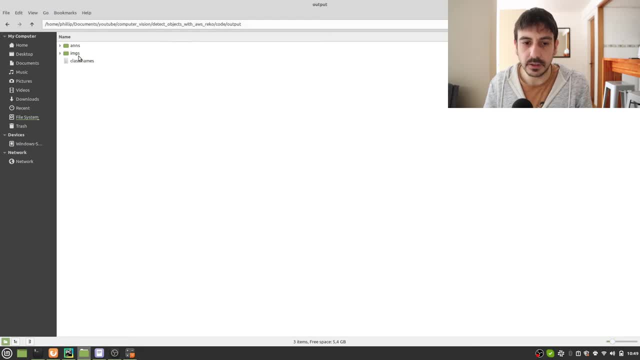 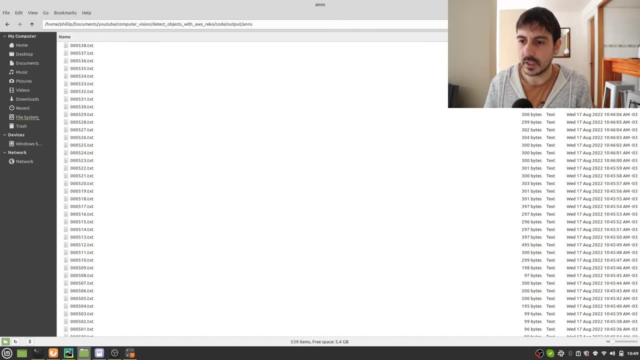 And also another thing you should notice is that if I take a look at, for example, the annotations and I order by modification date, you can see that the last one was saved 1046.. And the first one was saved 1035.. 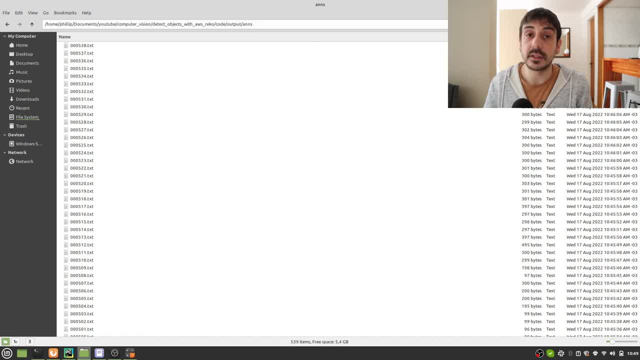 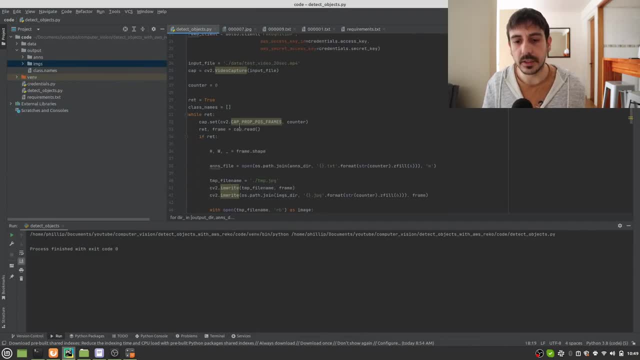 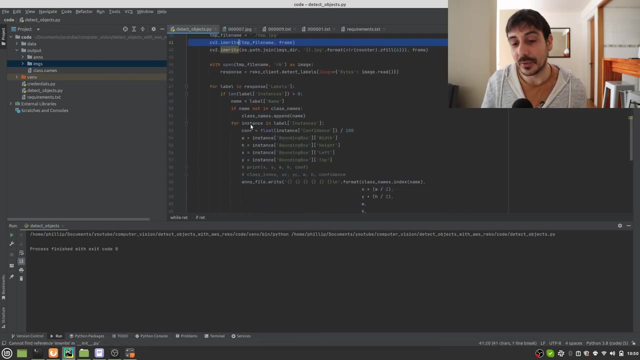 So it took exactly 11 minutes to execute the entire process, And, although we are doing other things in this script, we are also, uh, extracting the frames from our video and we are saving the image, uh, twice, Uh. so we are doing other things. 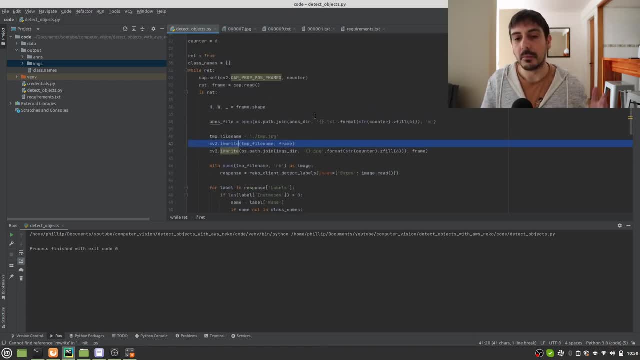 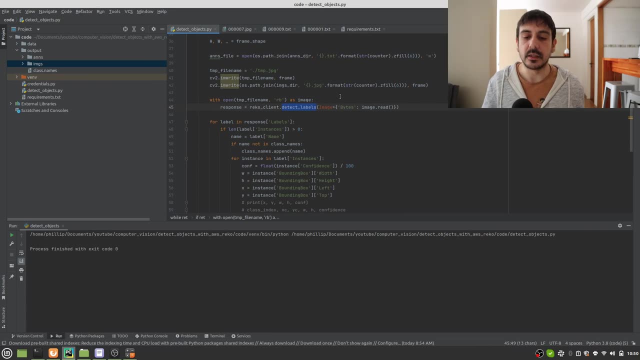 It's not like we are only executing record, but, if I'm not mistaken, I think the. every time we call This API, the, the uh, record detection. this is our bottleneck. This is where we are expanding, or uh, the most amount of time. 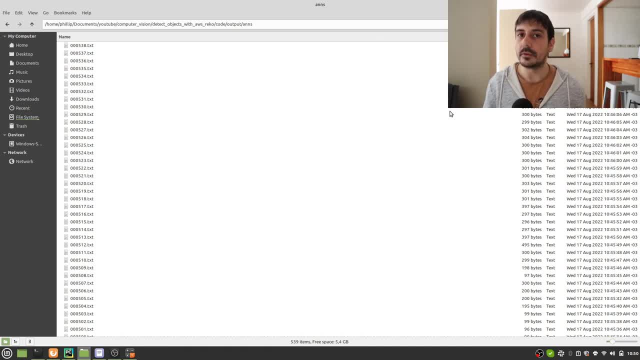 So, uh, it doesn't really matter if you are executing only a few images, but if you are executing a lot of images, please be aware this is going to be expensive because it's not a free service, and it's going to be expensive also in terms of computation time. 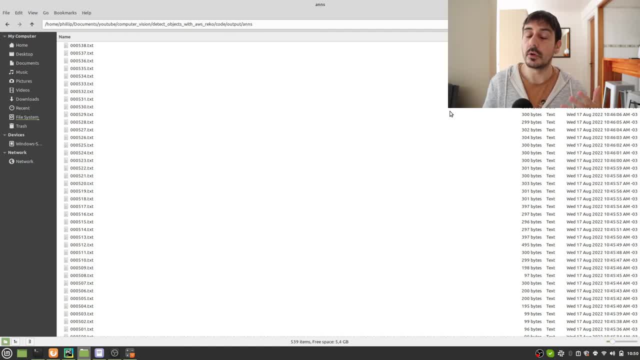 If you execute, if you build your Your own- uh, I green, your own, your own object detection- I green and you make it efficient. Most likely you are going to spend way less time than this. If you do something that's real time detection, for example, you'll be three or something like that. but these are only a few final considerations and that's going to be it.